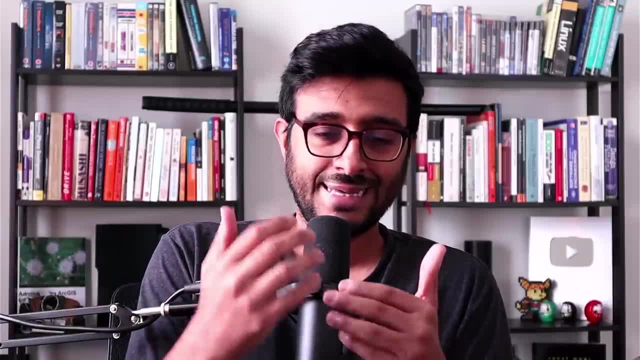 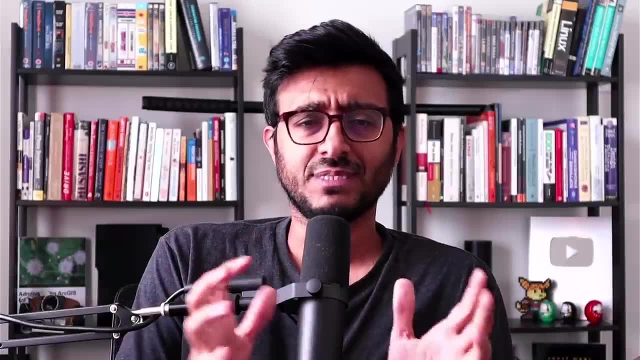 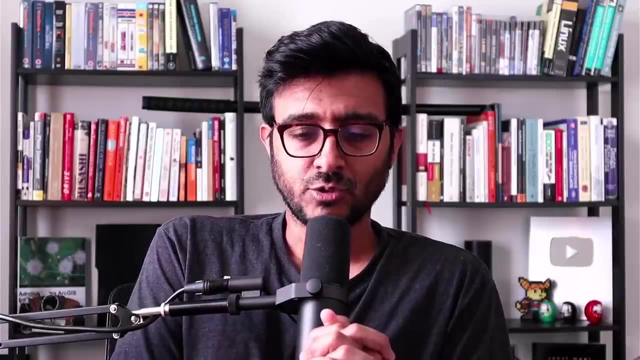 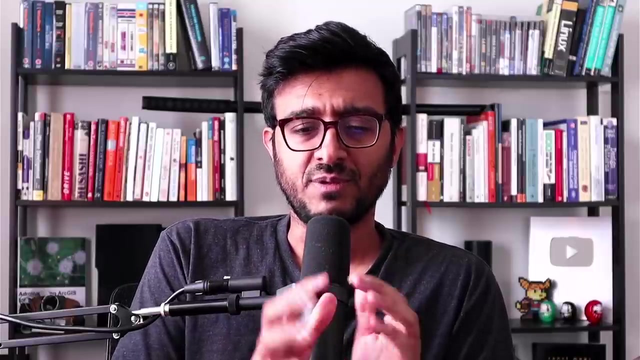 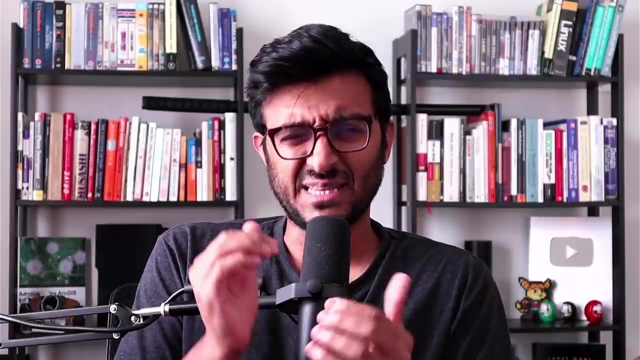 that uses graph things like social network, you know, networking in general- electric network, gas pipe, stuff like that, where, where you need nodes to be connected to each other. so in this, in this video, I'd like to kind of give my opinion about graph databases and how you can effectively build one by just understanding the 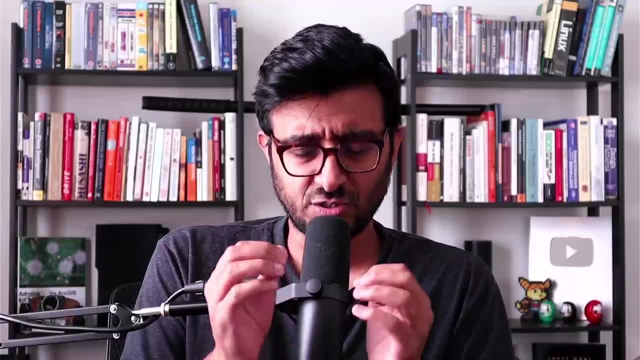 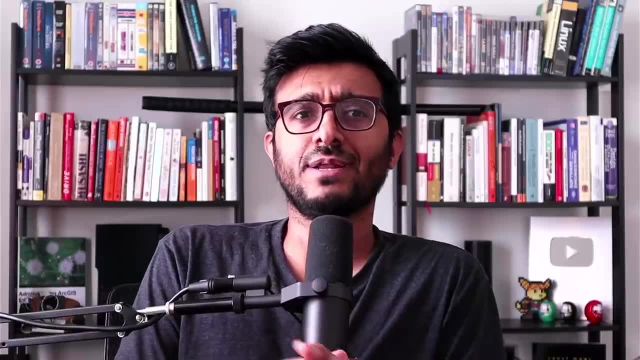 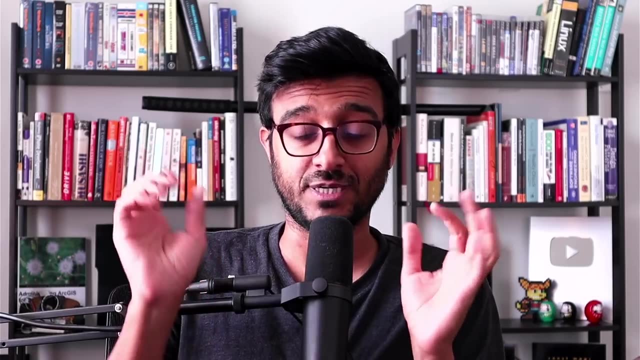 building block of an actual database. we start from there and we build up. let's jump into it. welcome to the back engineering show with your host, Hussein Nasr, and I actually recorded this video in a very crowded place and it sounded well in my ears when I used the airpods pro. 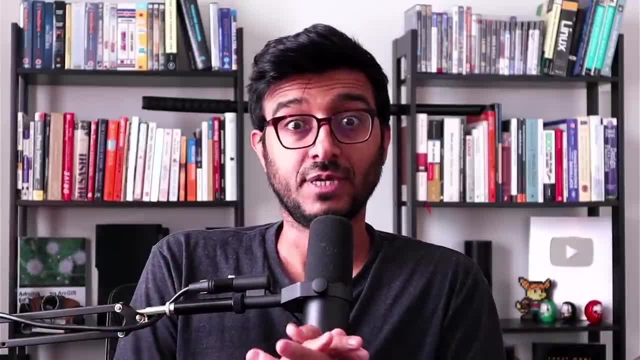 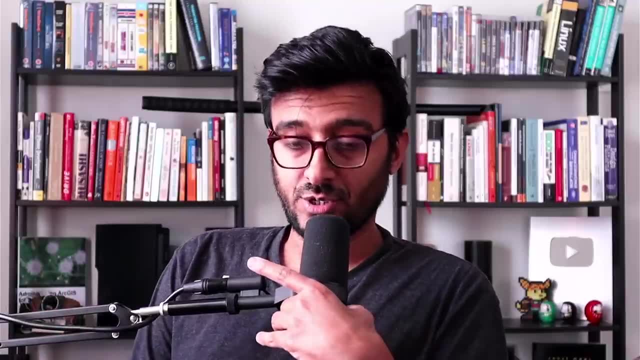 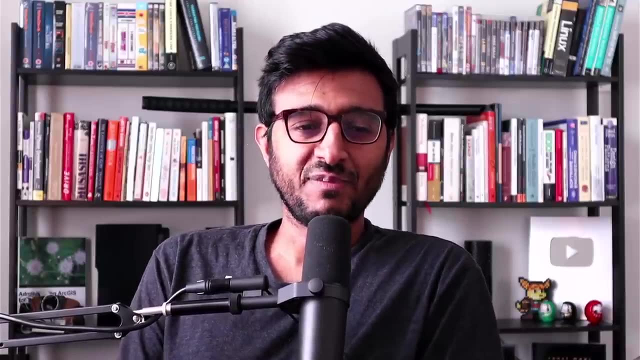 but when, when I actually posted the video from my phone, it actually you guys like yelled at me it, it turned out to be terrible audio wise, so almost not audible. so here is it again, hopefully clearer. so before we really talk about graph databases we really need to talk about 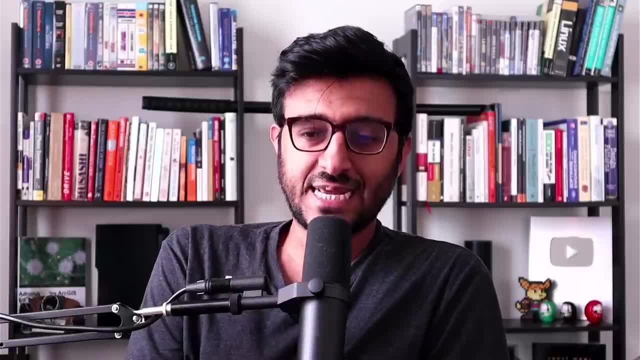 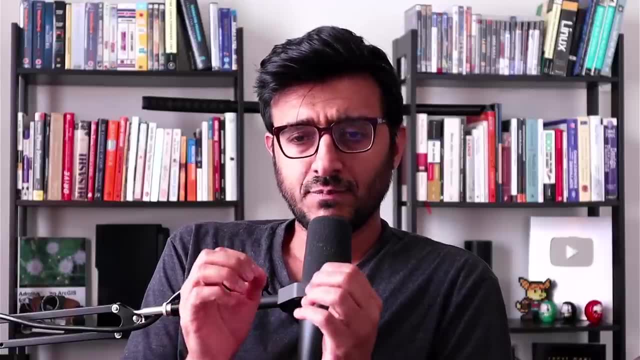 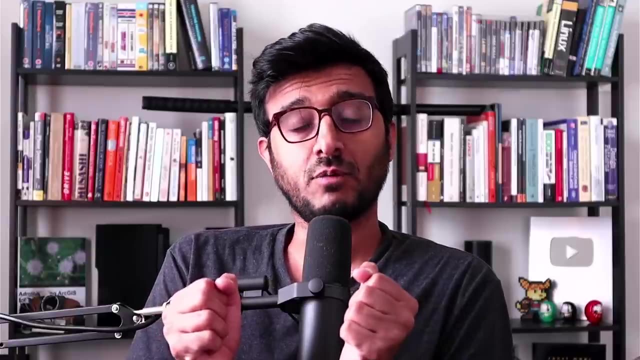 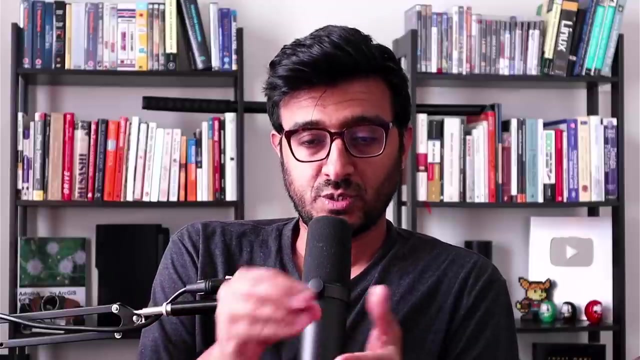 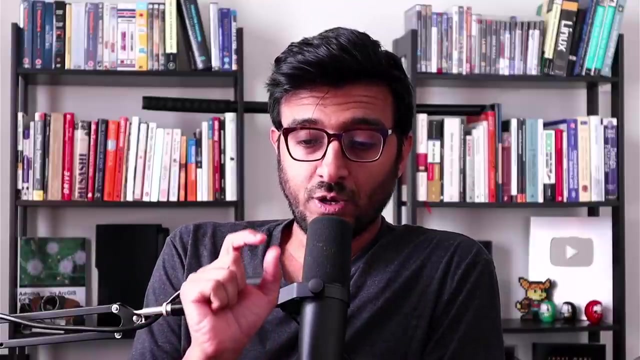 what is a database? the understanding of really what qualifies as a database is the critical. a database is a software that persists data to disk and reads data from disk in order to even pull certain information or search for a specific item right from desk. and this is what what it boils down to: the constraints that the database 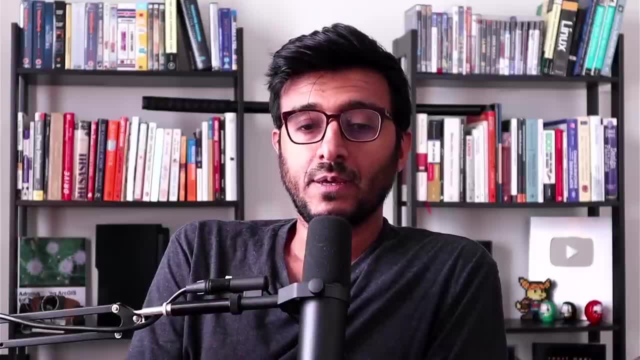 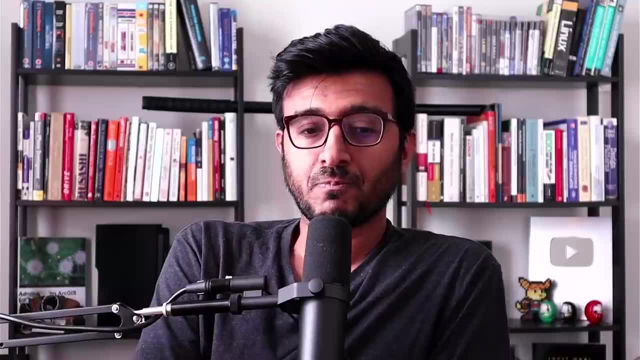 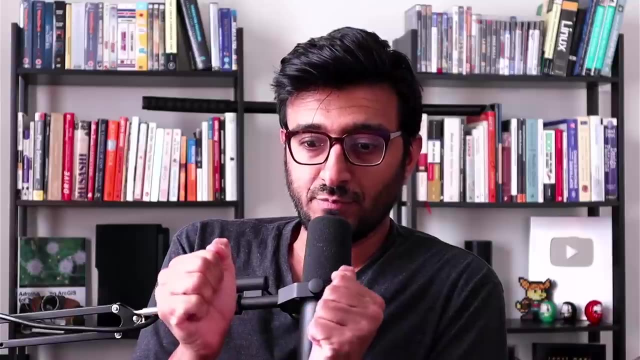 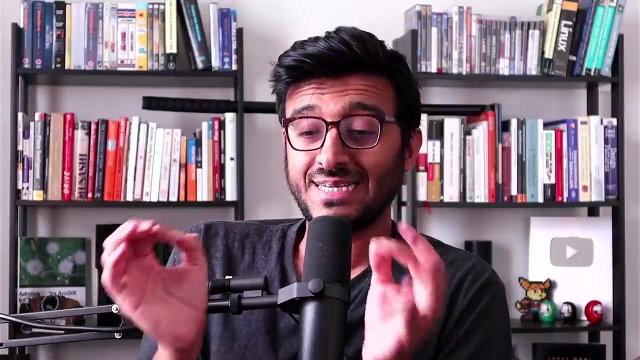 has to oblige by is the IO. the fewer the IO you make to disk, the faster your query becomes, and this is the limitation that we have we run into. so if I make an IO from this, I get a block of data, and if what I'm looking for is exactly in that block, then I have one. 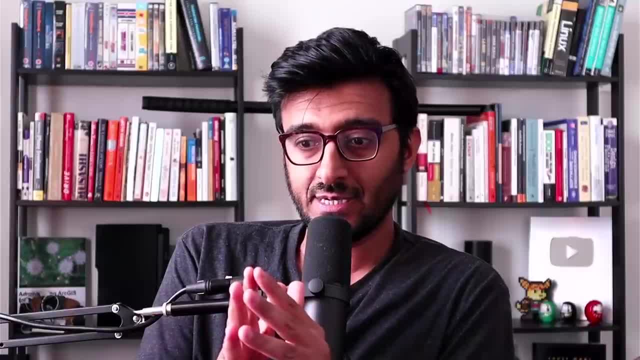 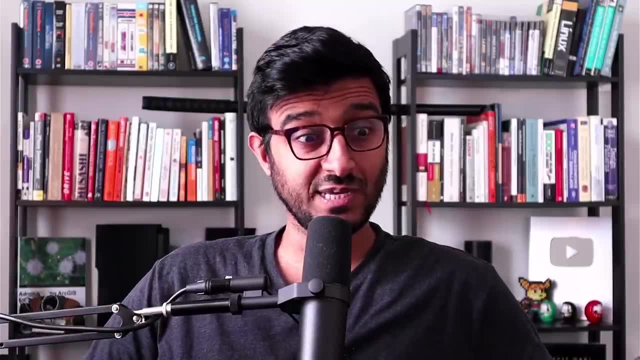 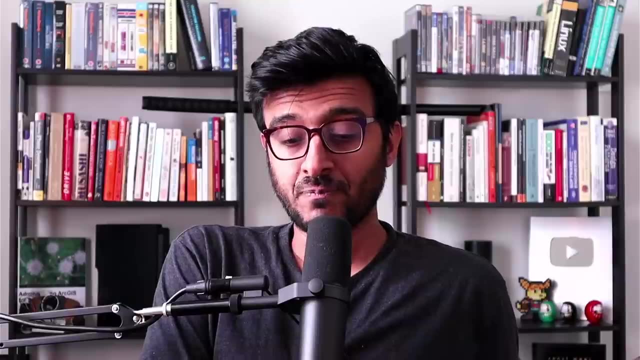 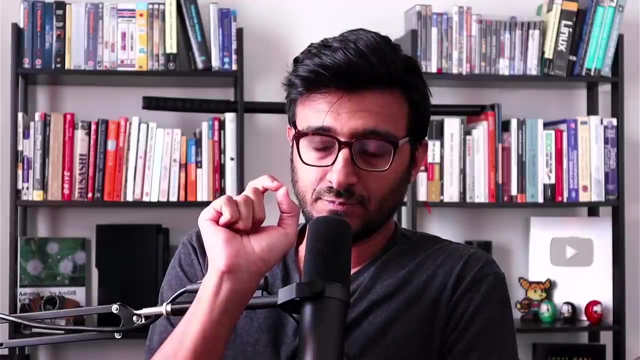 find myself looking for one thing- and as a side effect I'm issuing many, many, many IOs through the entire desk to look for this thing- then the the query will take longer amount of time to finish. this also applies to writing right. if I write a single value- and I wanted to persist that- 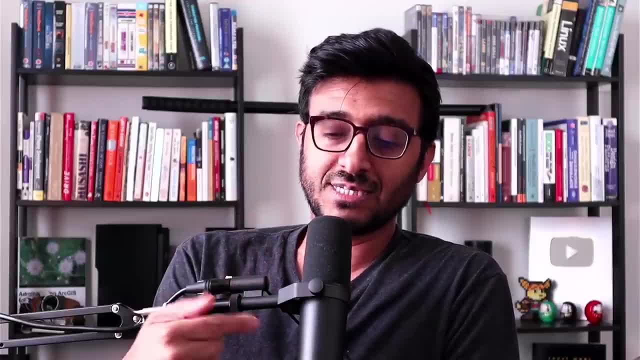 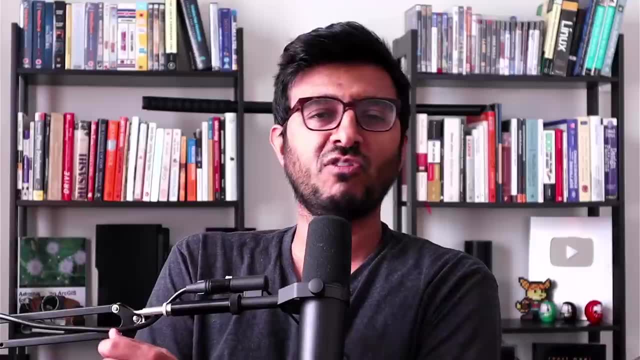 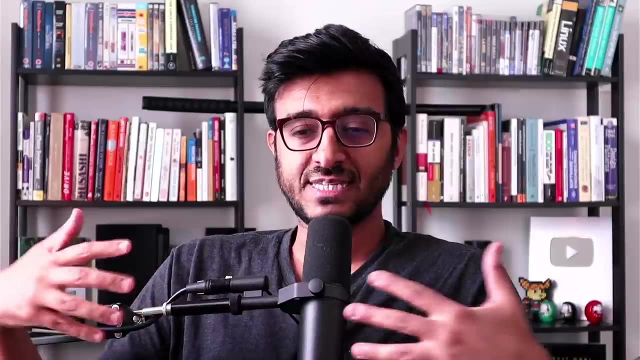 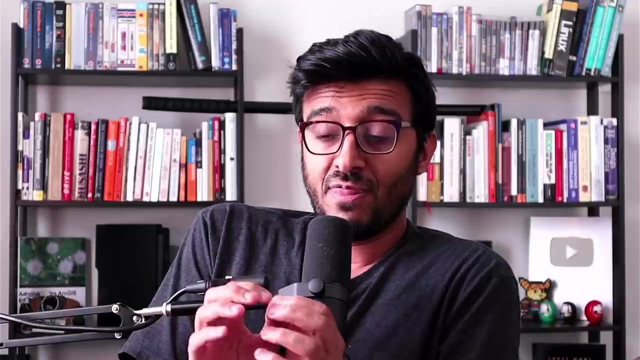 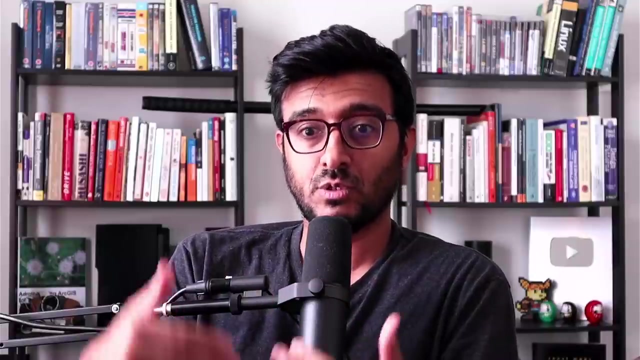 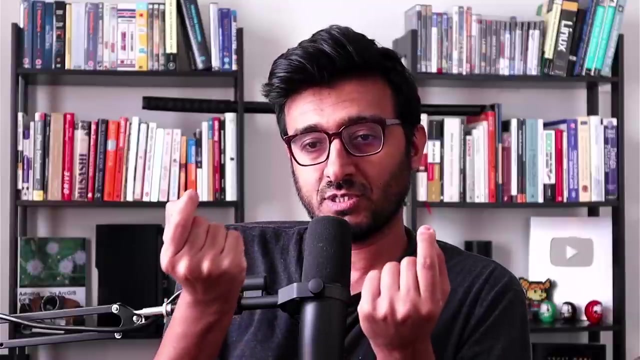 the amplification as a side effect of what the database does as a system processes, as a overhead. you know maintenance, storage, this amplification right. you know updating index structures, stuff like that. the larger the amount of IO that my write result to, the slower the right becomes, okay. so if I can write, if my right corresponds to a single small 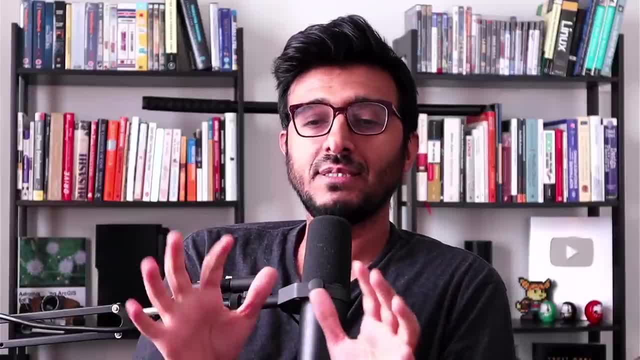 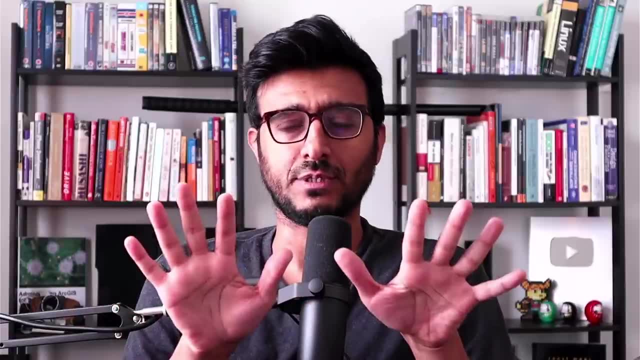 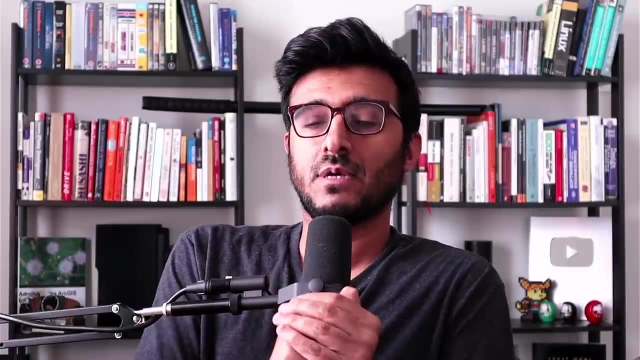 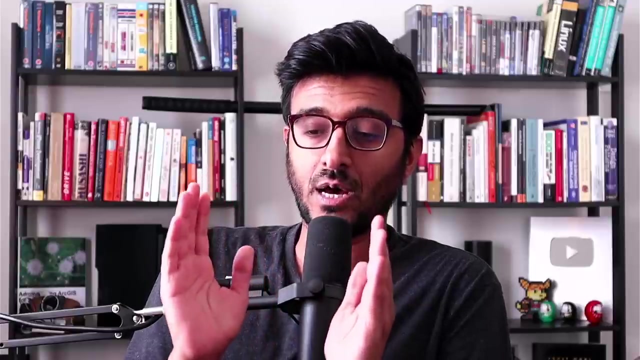 thing, then I have effectively optimized my rights, and this is really what it boils down to when it comes to databases. now, if we zoom out a little bit and I am in the database itself, I can play different kind of games right, because I can have to search for something. I not only rely on the actual data stored in desk, but I can build other. 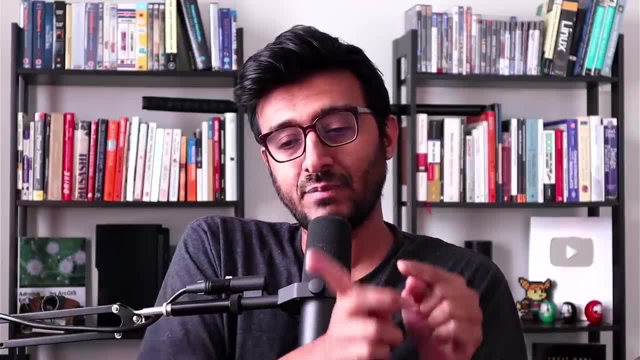 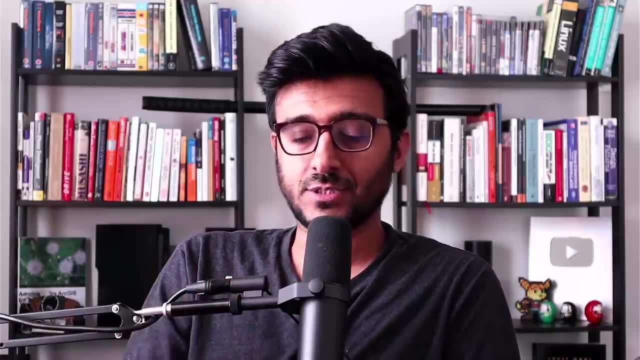 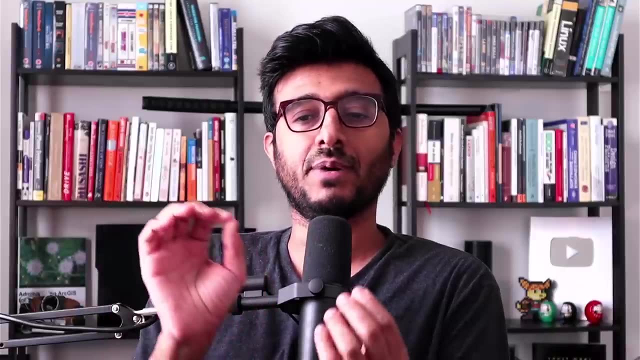 data structures that help me pinpoint where the data exactly is, and these are called mostly indexes, so the index is just like an actual index, right? you find in the secretary's office where, if you want to find a company by that that starts with the letter Z, you can find a company that starts. 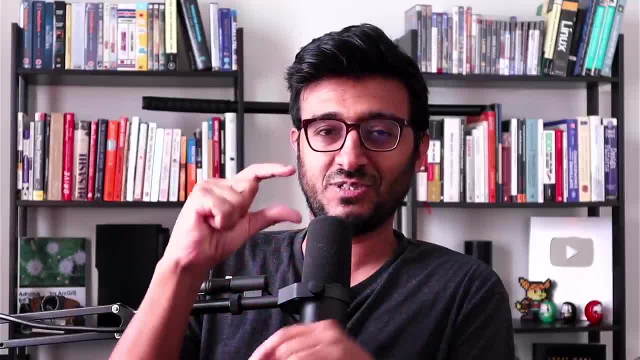 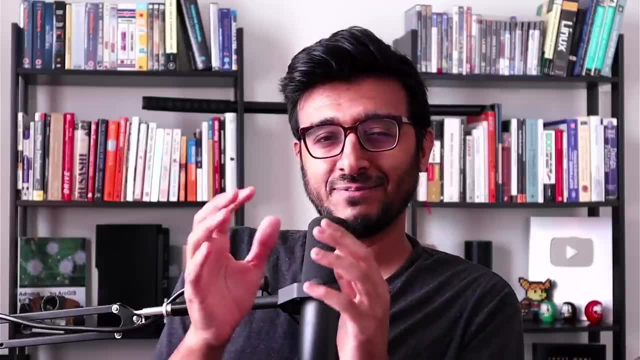 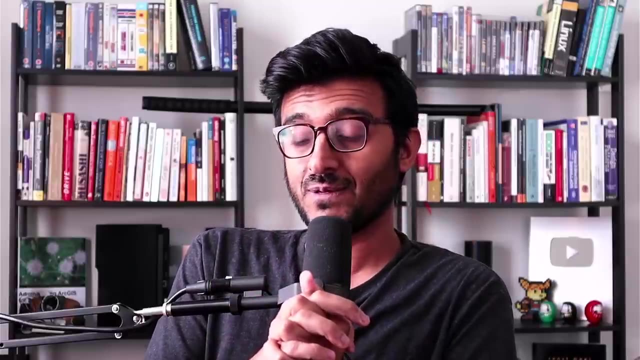 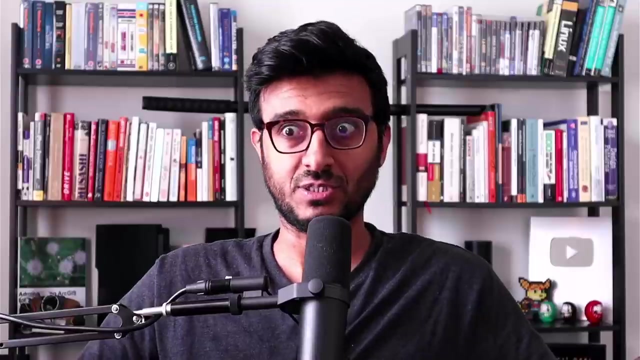 with the letter Z, you can jump to the section where the companies are Z's and then search only the Z's right or Zed's if you're from the UK, right. so that's effectively why it's optimal to use these external data structures, right, because it helps you pinpoint. oh, I just only need to search this portion instead of searching these all these other things. this results when: fewer IOs, fewer options. 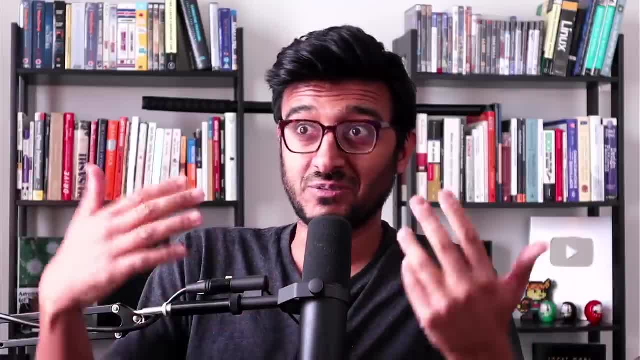 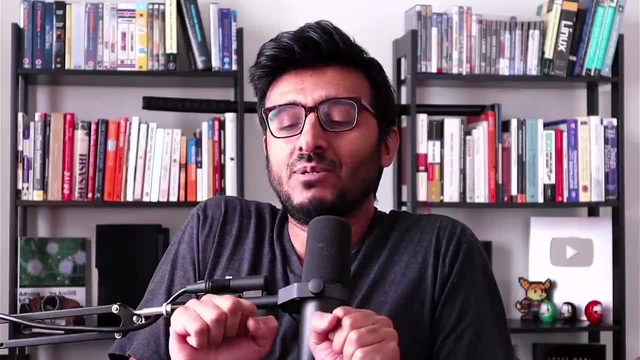 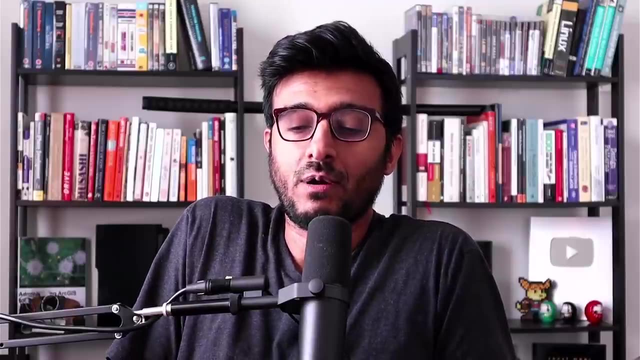 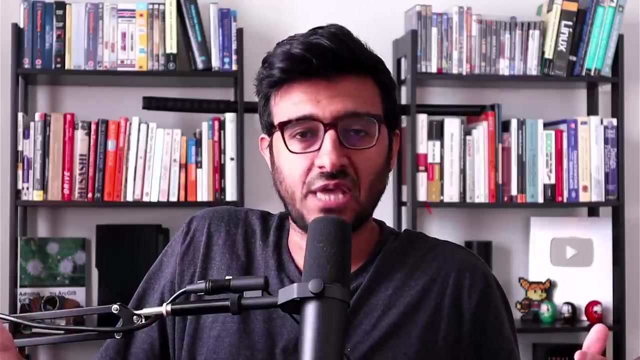 IOs means faster query and everybody wants faster results, obviously, like this is the goal, Once you understand this thing. now we need to talk about the storage engine right, And this is where the game is being played, where the classic relational databases store things in tables, rows and columns. 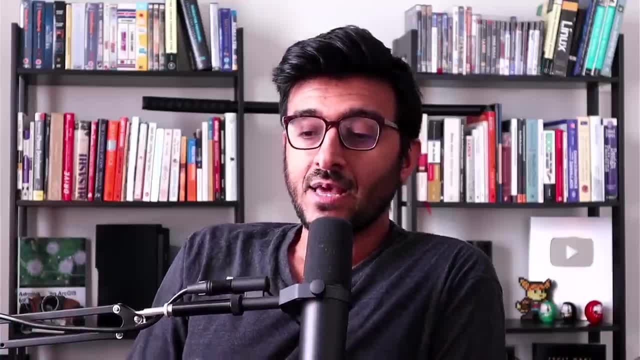 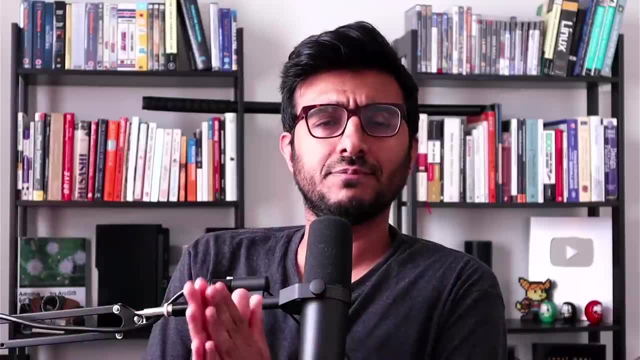 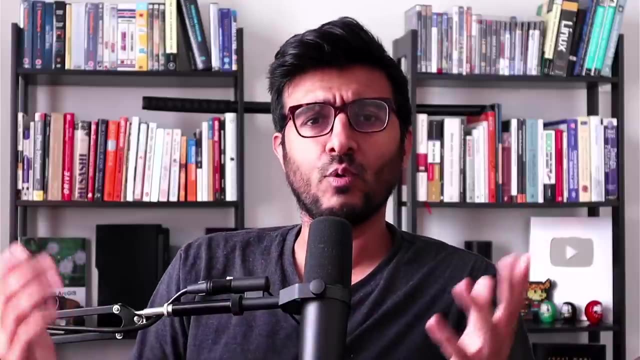 That's the classic things, And this was a general purpose design where, hey, anything you have just stored in a table And what does it mean really Table? what does it look like? So let's take a table called employees. 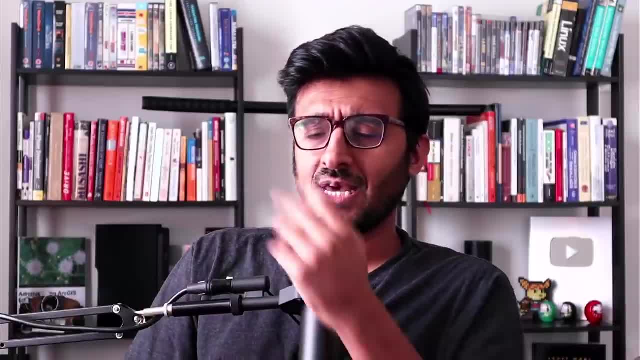 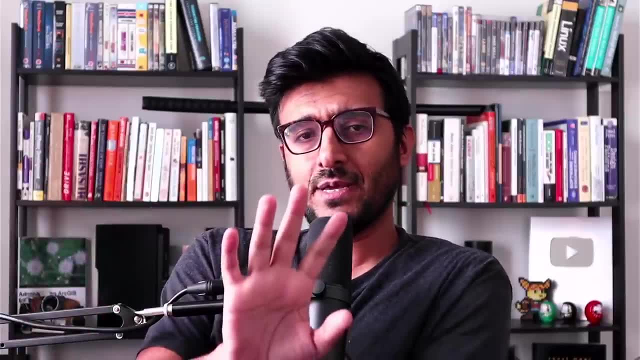 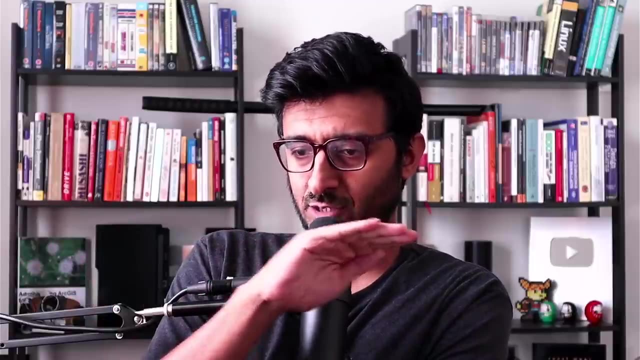 And you have an ID field and a name field and a salary field and a date of birth. So you can design a database to store. You can design a database to store these values in a consequent manner, so that every row is just following the other row. 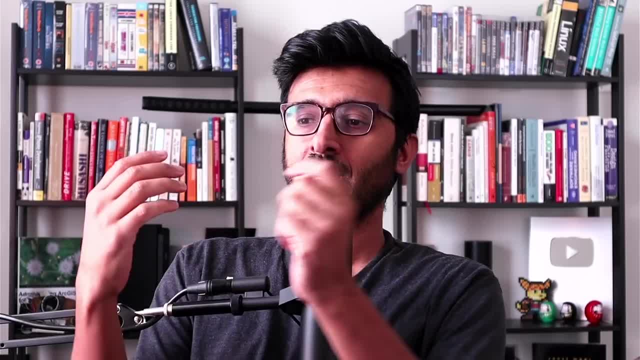 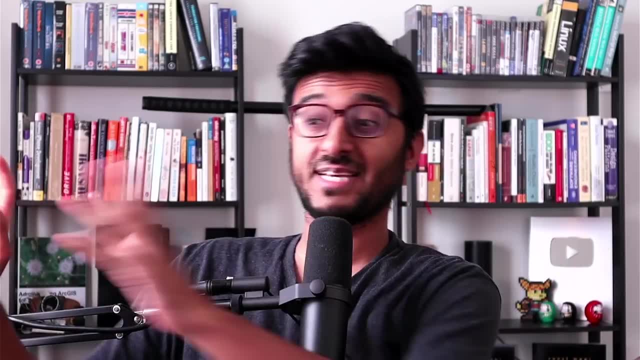 So I employee ID number one. his name is Hussein and his salary is blah blah blah And he was born in blah blah blah. And these aren't just a number of bytes. And then the second employee just comes exactly after it. 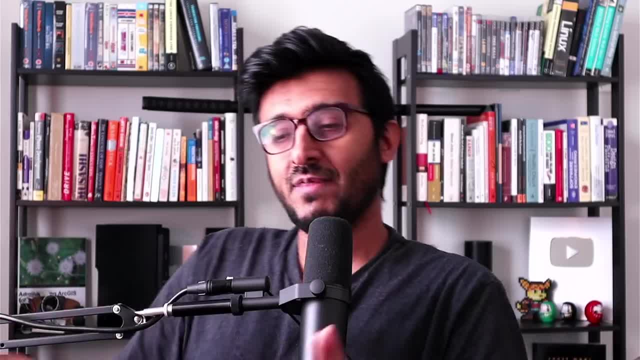 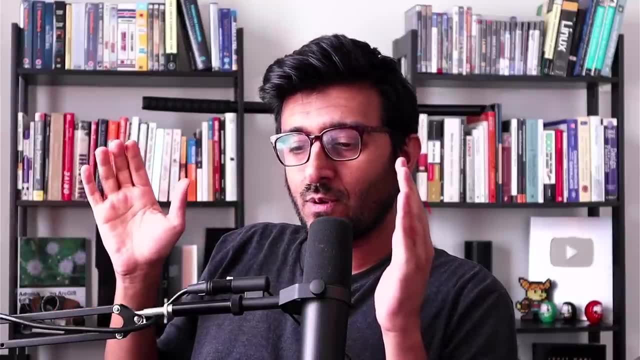 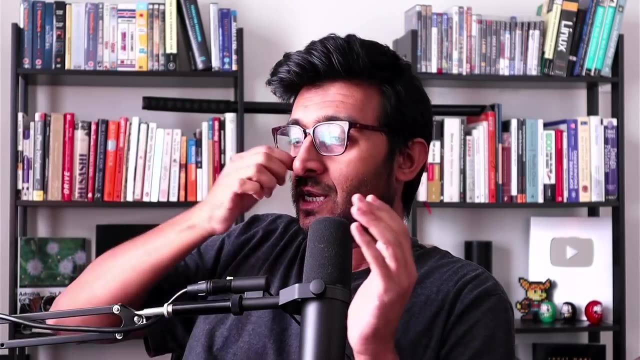 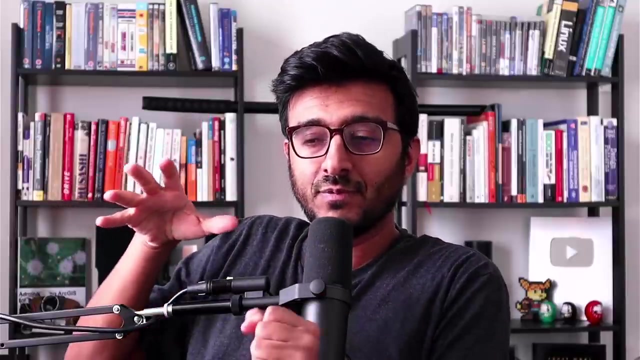 Employee number two. his name is Adam blah, blah, blah, blah blah. And then you have a string of Bits, right? So think about this: This is called a row store. You're storing per row. So if I have an IO, if I do one single IO, not only I'm going to get one row, but I'm going to get multiple rows from this single read, right? 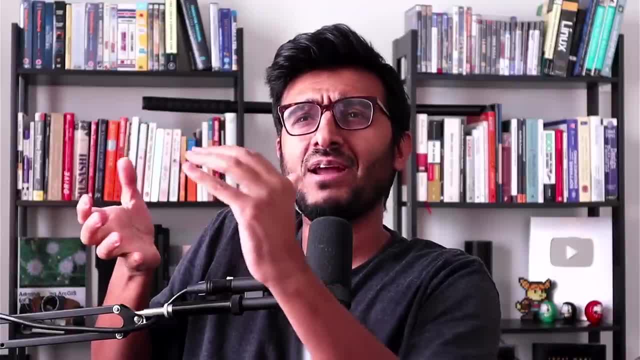 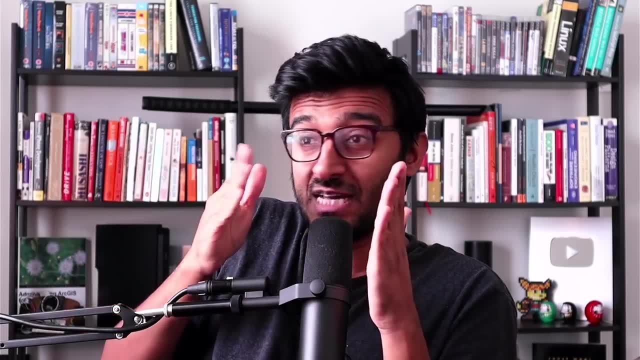 And logically, if you think about it, how can I fit Many rows in a single IO? Well, you make the rows smaller If you rows have, if your table doesn't have many columns right, Or it doesn't have like long. 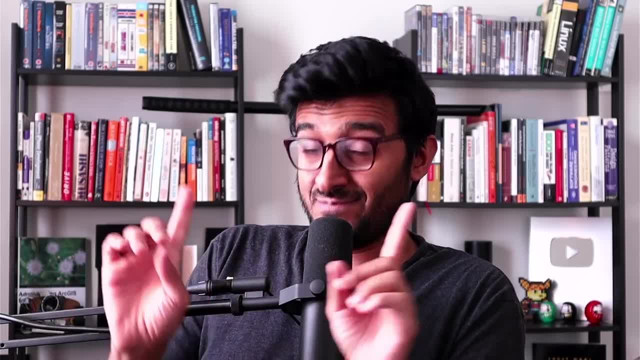 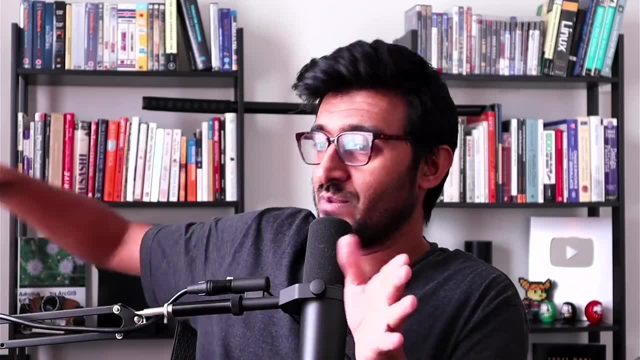 So if you have values like strings, long strings- if the database decide to store the string in line- by in line I mean in the row itself- then the row becomes so large. That means if I have a single IO, I get very few rows. 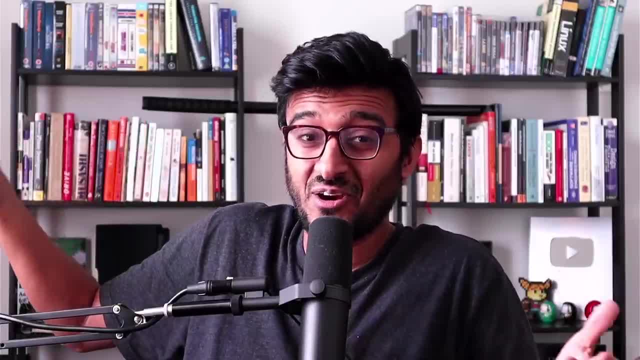 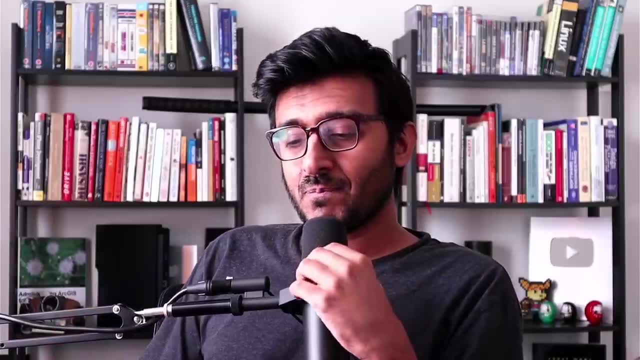 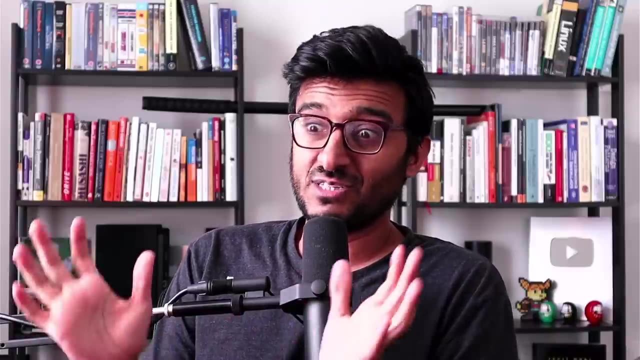 Because The row cannot fit in it in an entire page. This is how databases read things and logical pages. So, By the way, this is not entirely correct when it comes to strings like. Postgres, for example, doesn't really store like if you have like a whole document of a single string, right. 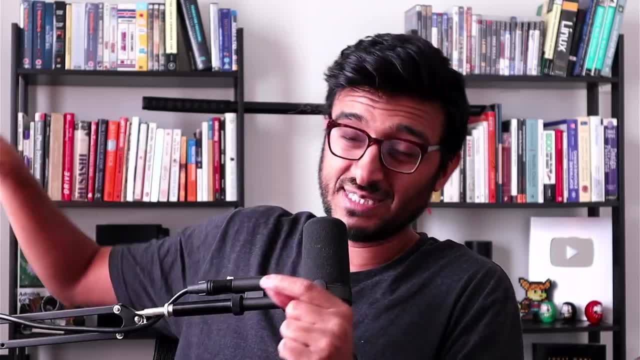 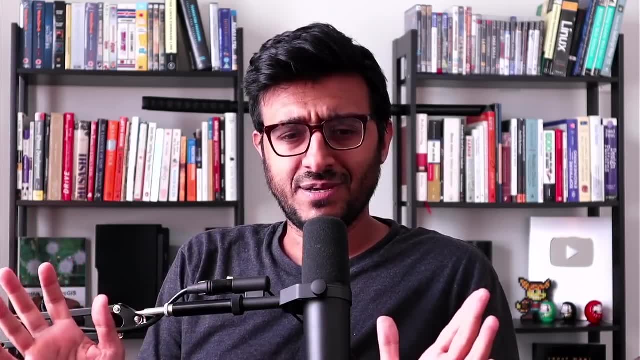 It doesn't really store it in line row stores that, compress it in an outside table and then Points to it in the row, right, But that's the logical thing, right? So now, if you think about it, so this, this use case, is pretty good. 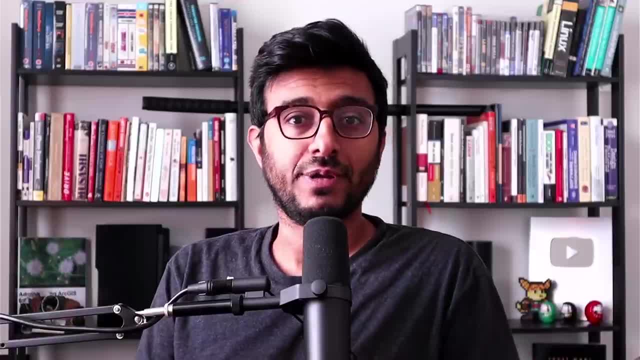 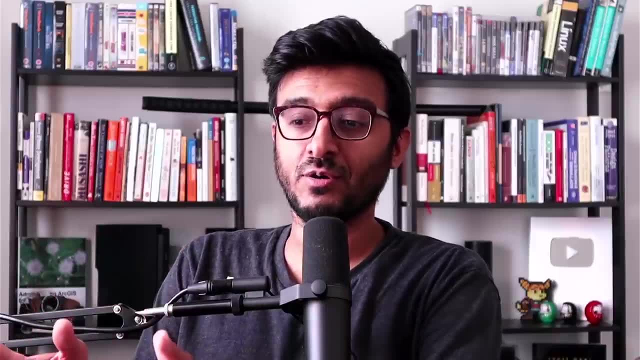 If you're like searching, you're displaying all the data, right? Hey, I want to display all the rows right And in a in a UI. so you want to do one IO and the the more rows you have, the better right. 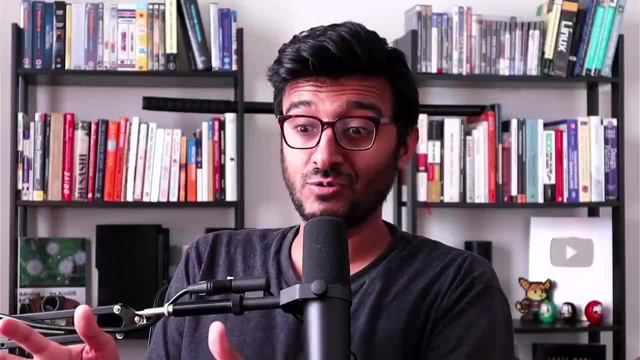 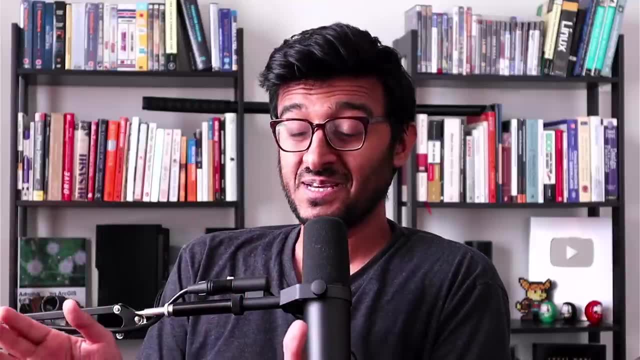 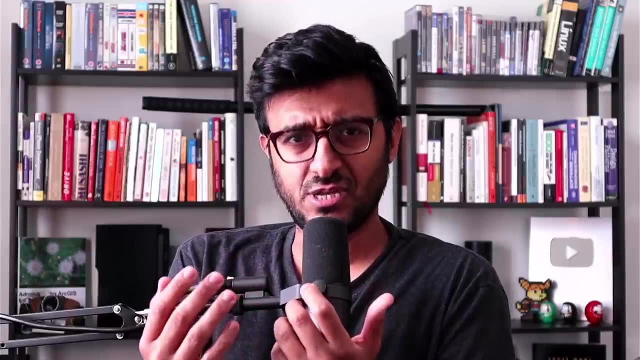 And guess what? This IO, you're going to give you all the rows, The row and all its columns in that particular case, because that's how you store it, Okay, So that's how it's optimized to Right. So some other people decide it's like: okay, this really sucks. 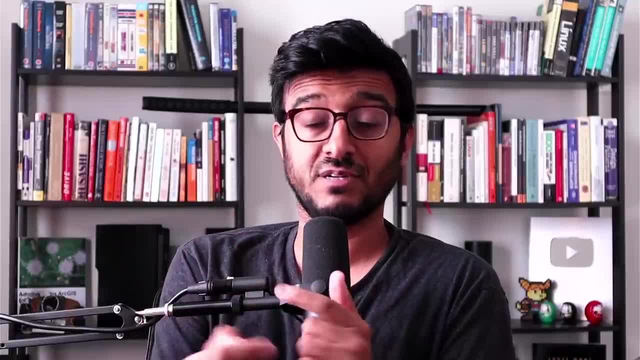 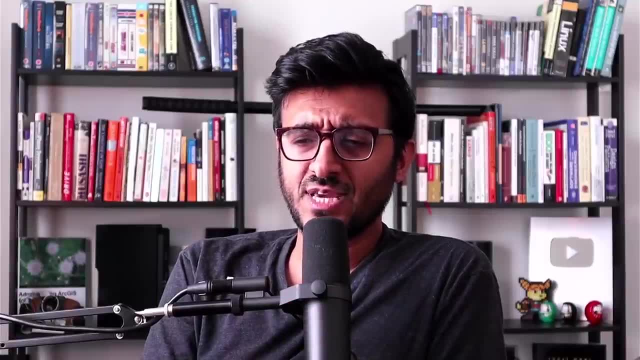 For other use cases. See, when it comes to use cases, every time come everything back, comes back to use case. So for that particular scenario, if you have another use case to like I don't know some, all the salaries. 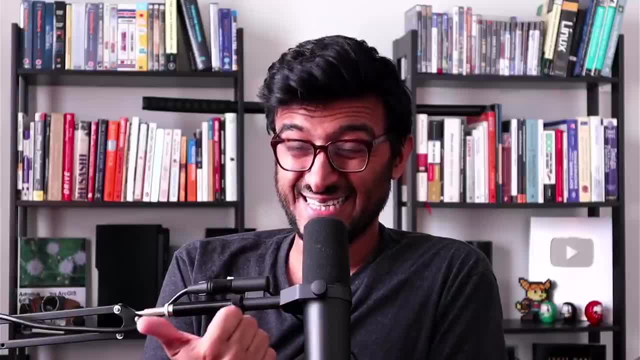 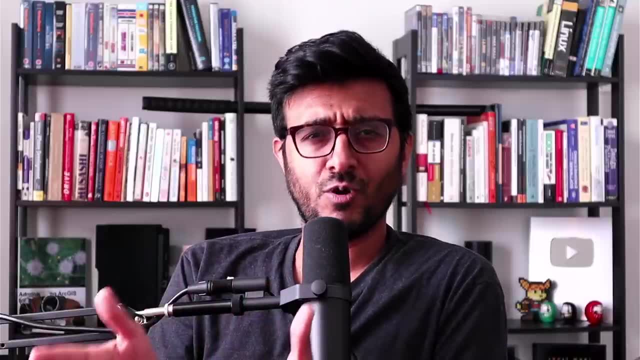 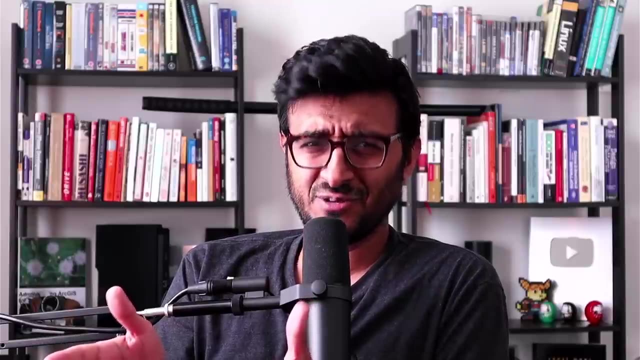 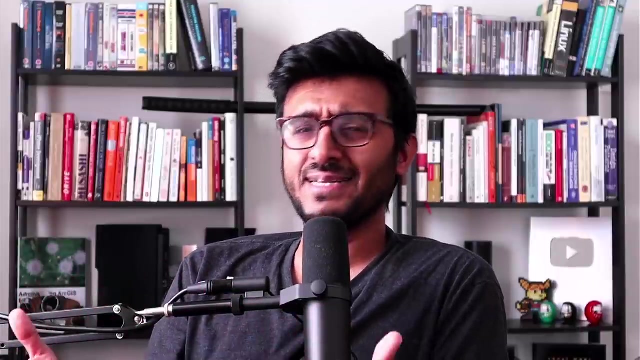 Then This particular use case is actually not very optimized. Why? Because a single IO- Yeah, It's going to give you X amount of rows, but you really just need the salary from the row, Right? So if you do that, then you're pulling the ID or pulling the name, you're pulling all that stuff unnecessarily and you just need the salary. 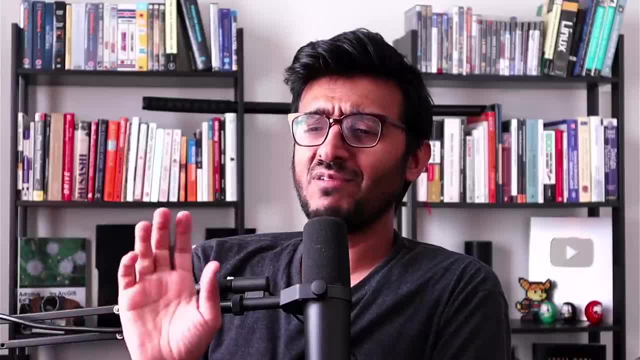 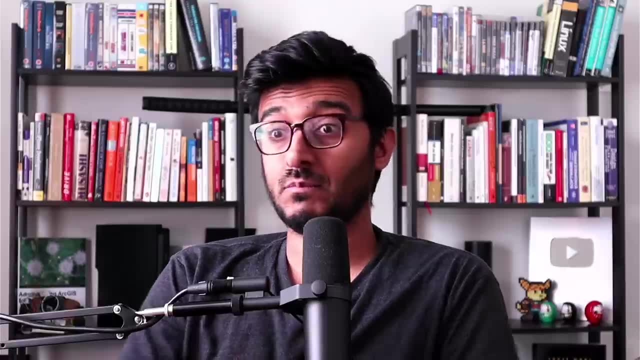 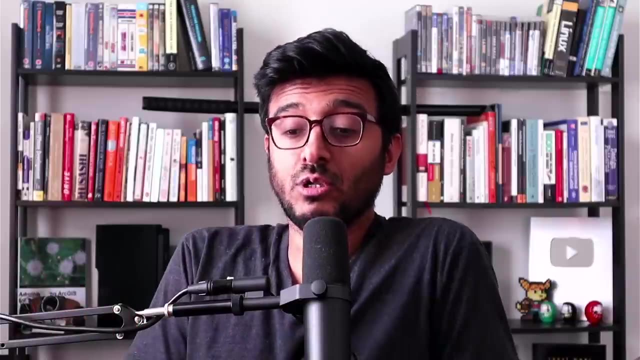 Right. So people thought about: okay, what? Okay? Okay, So if I actually store the table column first and the column in our databases was burned, so we had the row base databases, we have the column in our databases- or column stores, they call them where, Hey, store the columns, right. 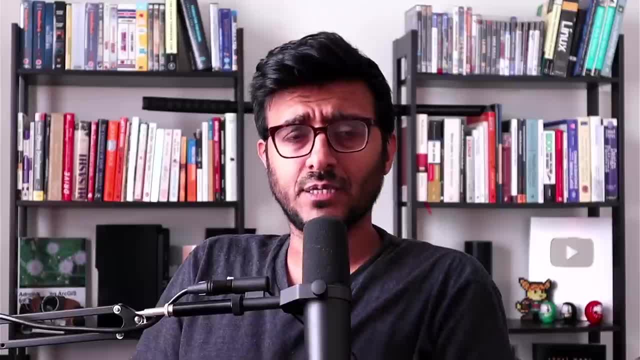 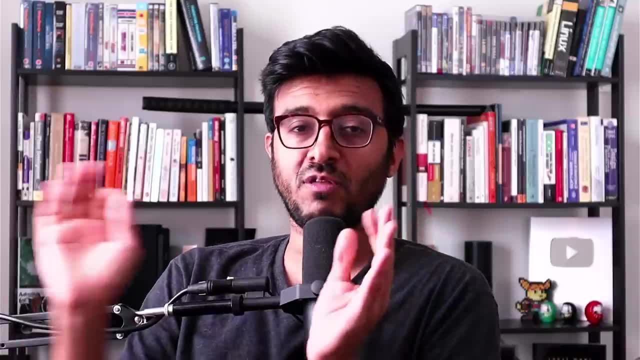 So it's column by column by column by column. So ID, let's say, store the ID field, store all The rows, all the values in the table for this ID. So ID 1,, 2,, 3,, 4,, 5,, 6,, 7,, all of them. 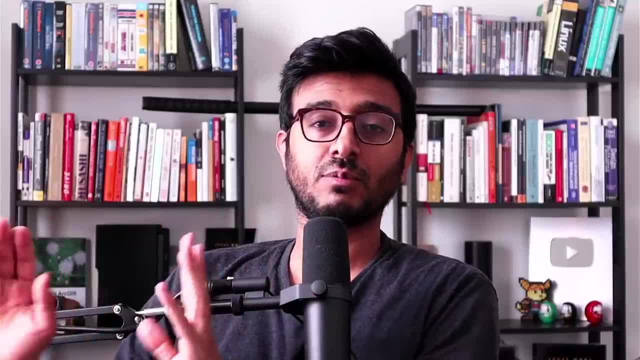 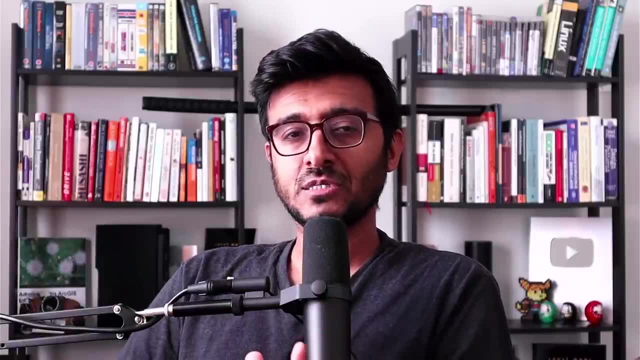 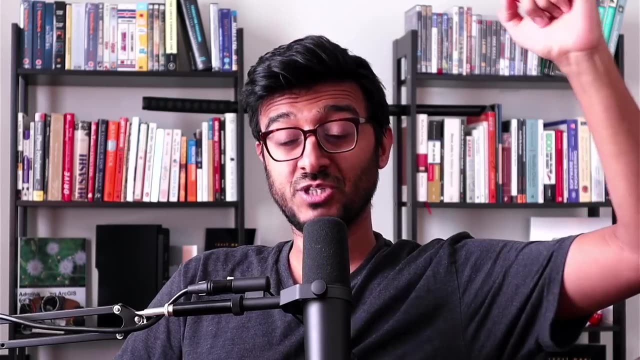 And then Store the names Hussein, Adam, rec, and then store the salaries next to each other: salaries 2000,, 3000.. So, and now you have a clear pointer of where the columns start. So now, if you want to do a sum, you just go to the exact page where the salaries 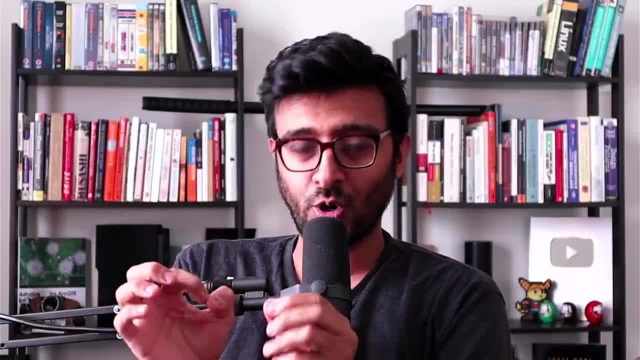 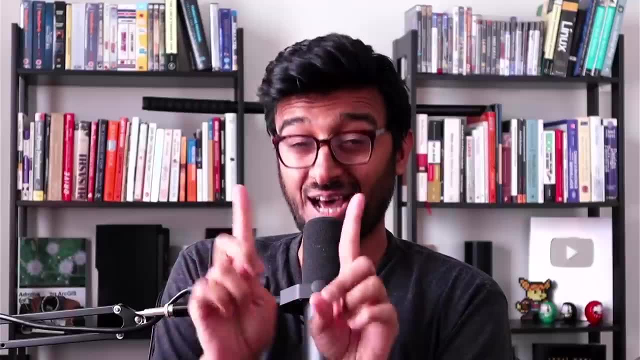 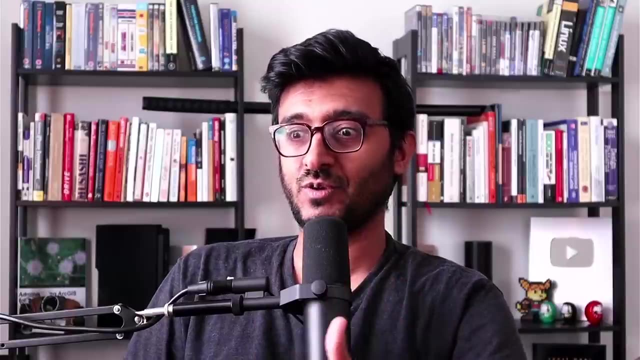 Column start and then do an IO And boy, this is optimized because a single IO will only give you salaries. So a single IO will give you so much salaries compared to the row store, where you a single IO will going to give you junk that you don't need. 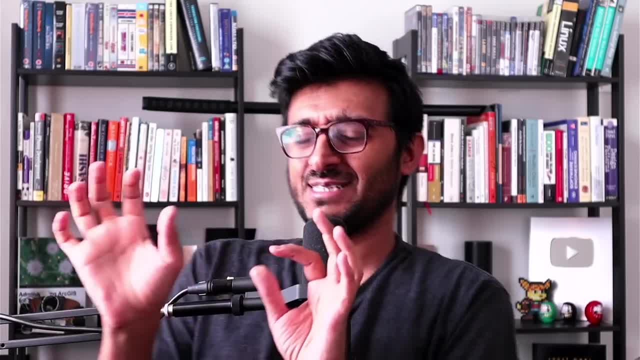 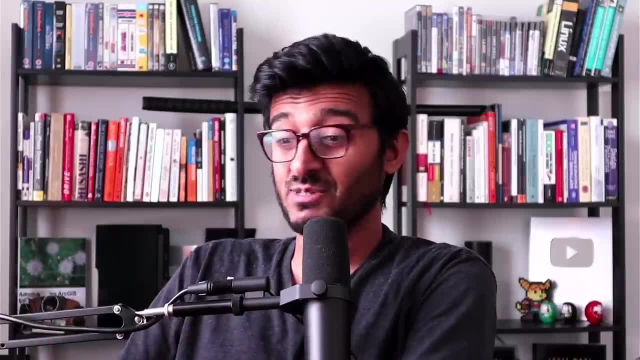 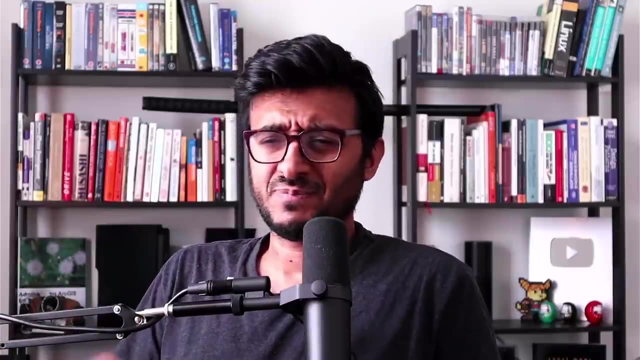 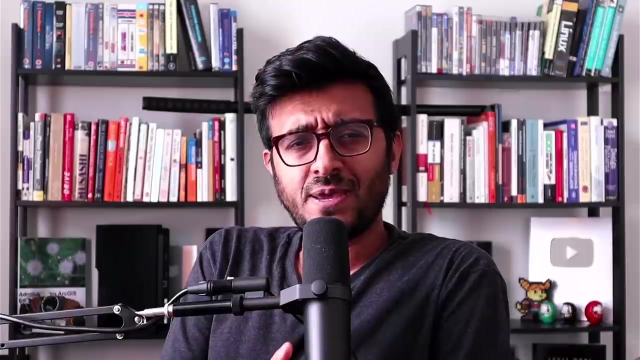 And even if you do select, start select salaries from a table. if it's a row star, row store, then Okay, Then it's still. the IO is going to pull everything and then only pull what you asked for. There are some optimizations. that database does like it doesn't have to hydrate that data structures and stuff like that, but still so that's how people think, right. 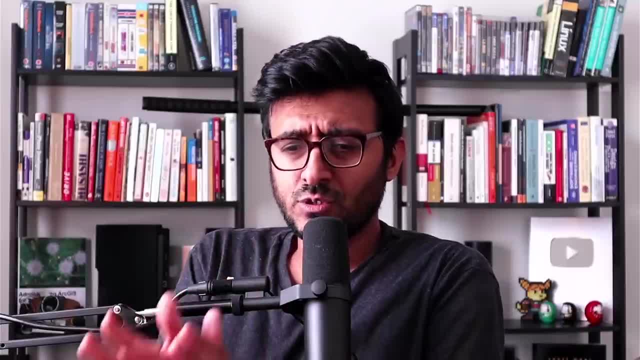 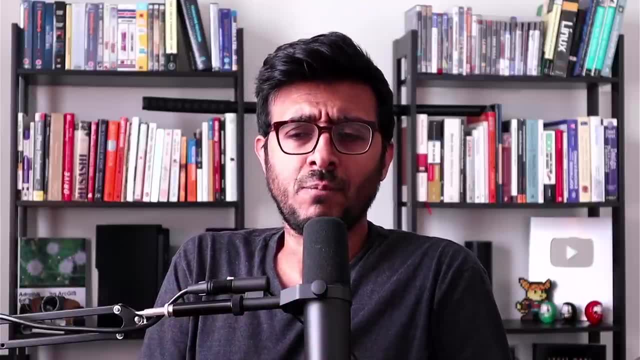 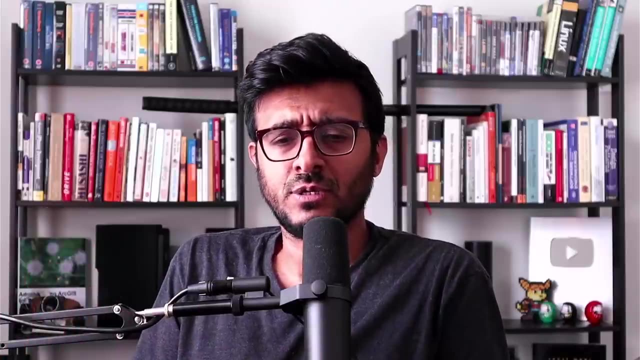 I know we didn't jump into the graph databases yet, but we have row store, column store, document. similar thing. Like I don't really need to store rows, row store, column Store, column store. So they build up their own binary data structure, right? 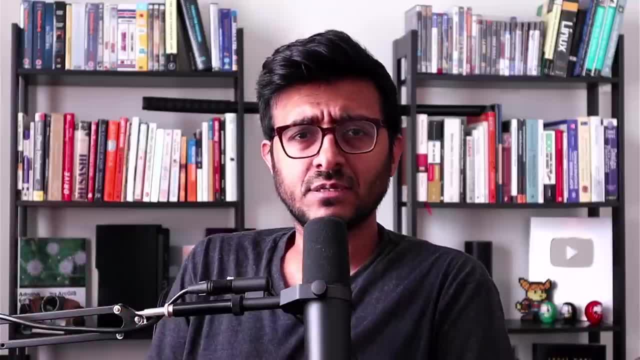 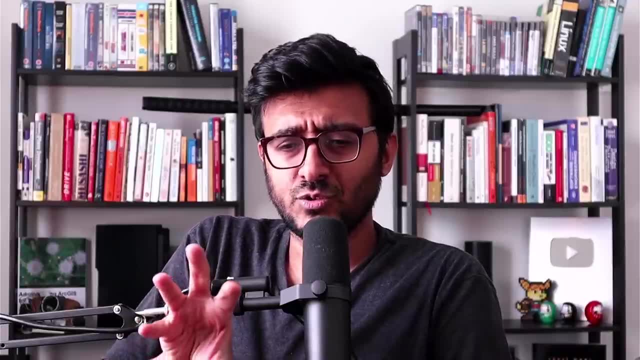 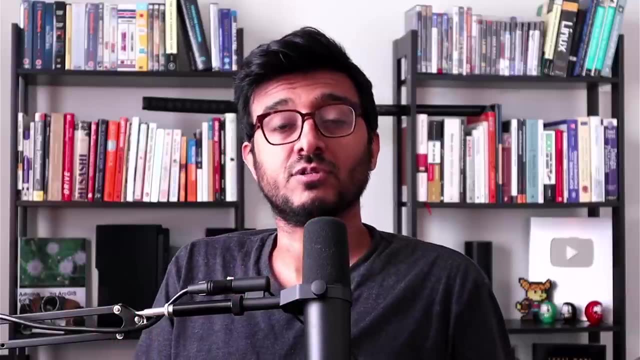 And this is how they going to store the data on desk right. So you, you optimize the storage engine based on exactly what you want to do. And now, while I don't know the internals of a graph database like Neo4j or or Arango DB, whatever they are- 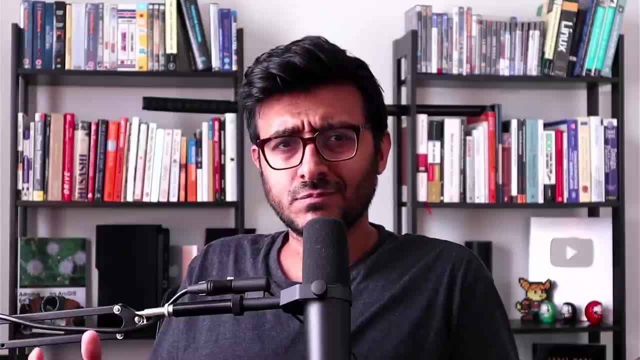 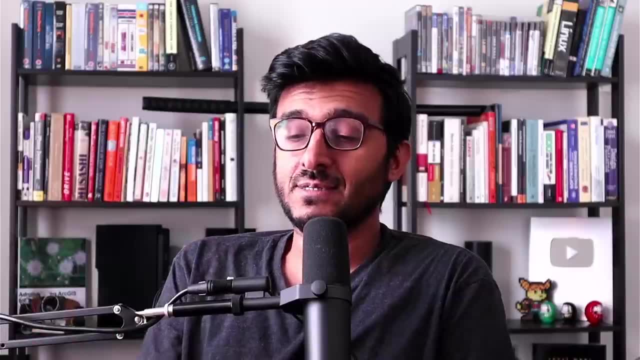 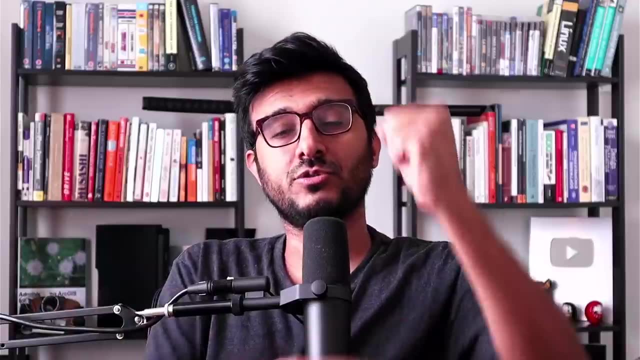 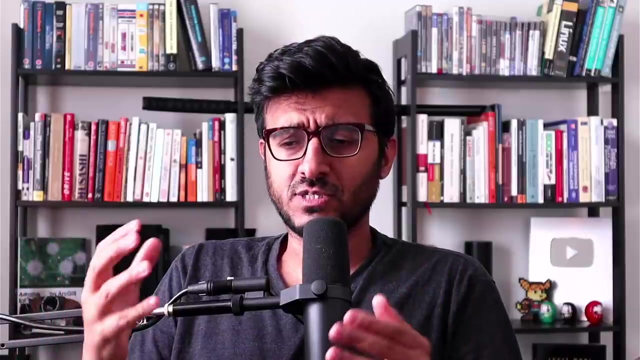 Okay They are called. think about logically what is a graph database? A graph database is a graph use case is when I have a single node I want to find all its children or all its neighbors, All right, And there are many ways to search for specific thing in the graph, right? 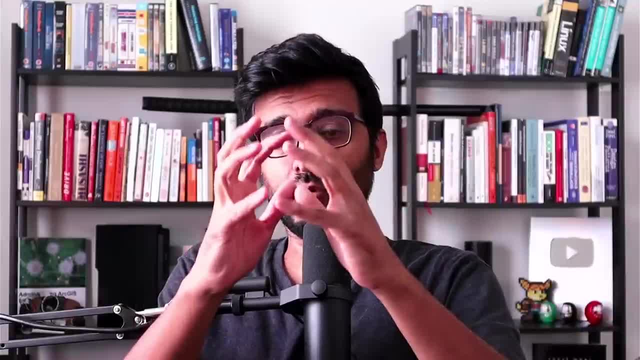 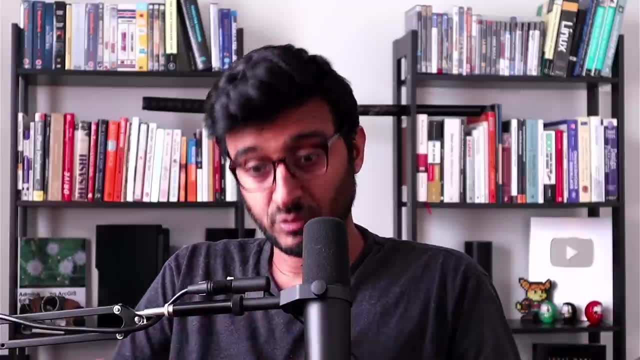 You can do a bread first where you say, okay, No, it gives me all your children, Right. And then, for every node, give me all your children. for every node, Give me all your children. That's a bread first, right. 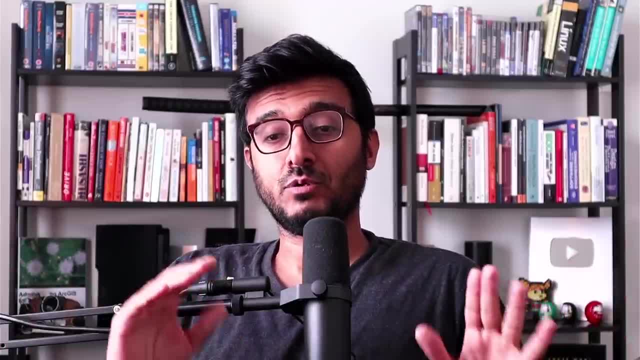 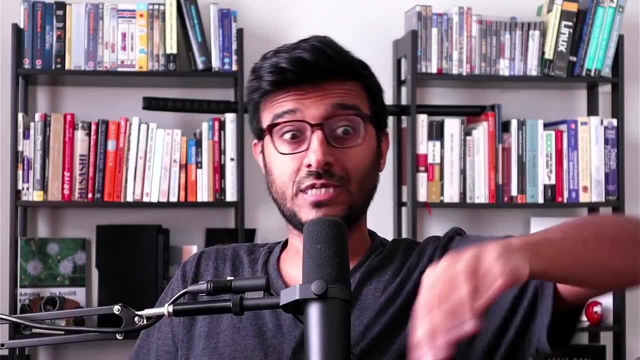 That's a way to search, And the other approach is the depth first. Well, okay, Give me your children and go to your child. No, don't give me the second truck, Give it. go to your child and give me its child, and go to your child and give me its child. 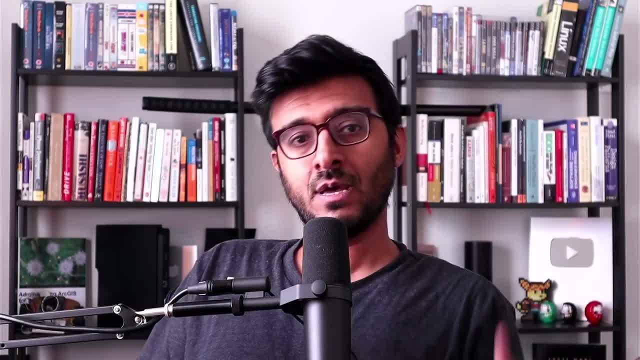 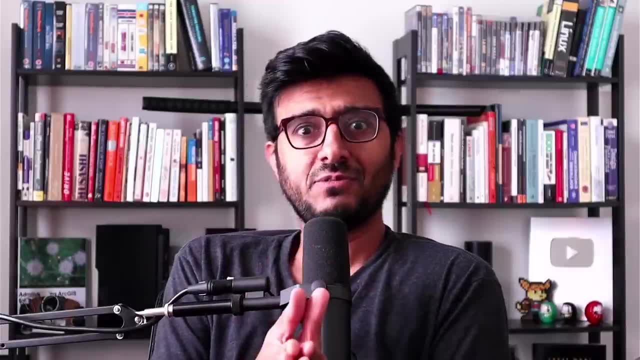 So you go in depth first and then you go back forth and there is pros and cons, There is no. Okay, That's the right way. It depends on what you're trying to find And based on that you can think we're saying: why do I need a database? 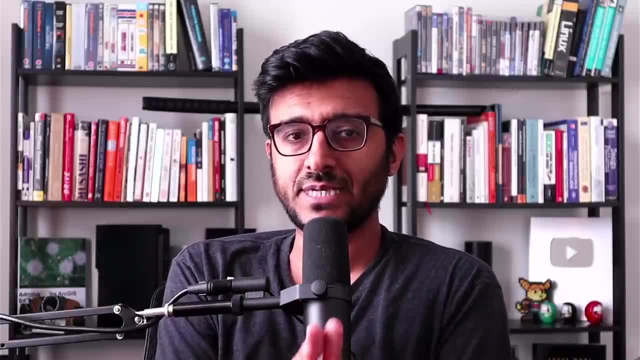 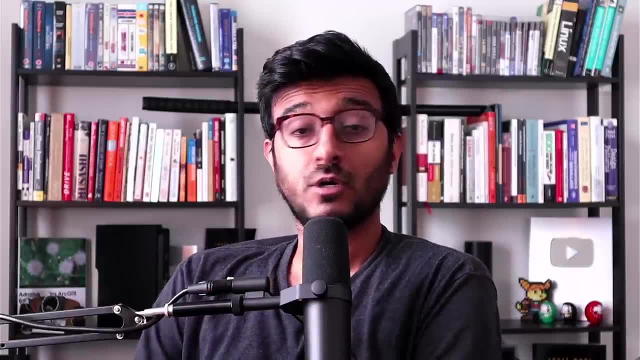 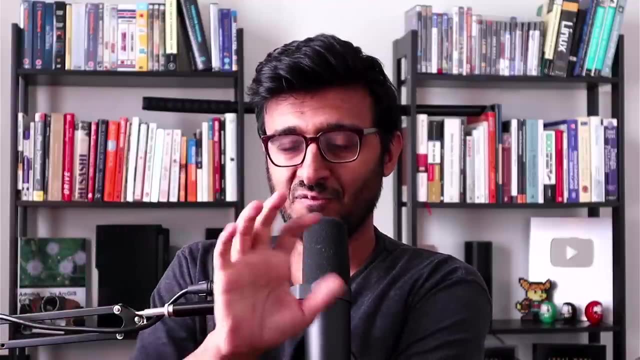 I can build a graph, use case social media using a relational model. Of course you can. of course you can, you can definitely do it, but will it be optimized for the search? Because, think about it, If you want to, uh, like Facebook, right? 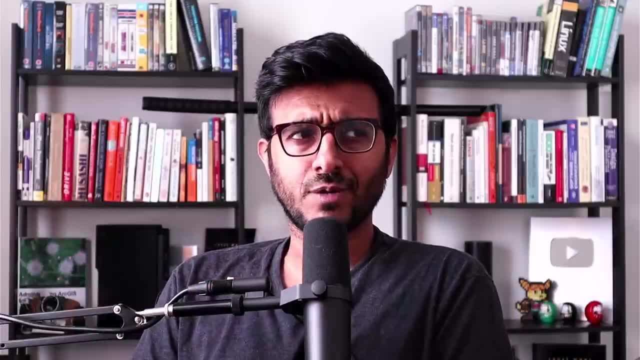 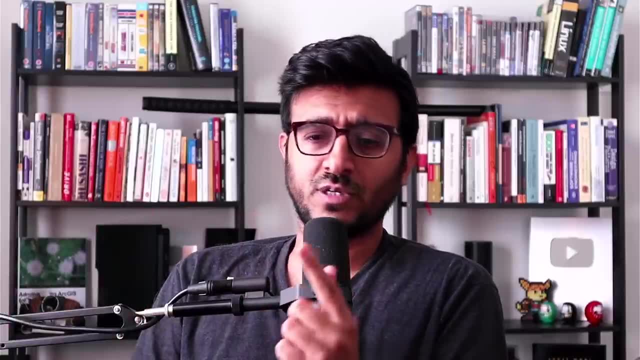 I am. I want to find all my friends, right. What does that mean? All my friends? you can store them in a table and say: okay, this is my friend, One is a friend of two, one of friend of three, one is third, friend of four. 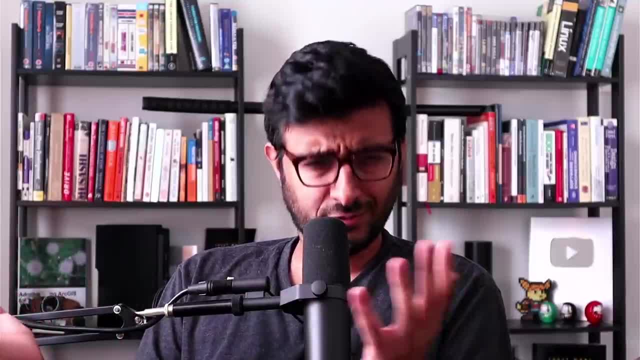 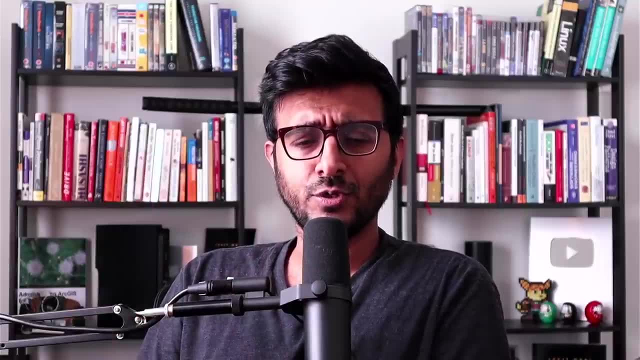 One is friend of four or five. So you, this is how you store it, right. This is one, one way you build a table and then you build a mapping, effectively right, And then, when you do that, you can store this even as a column store or a row store. 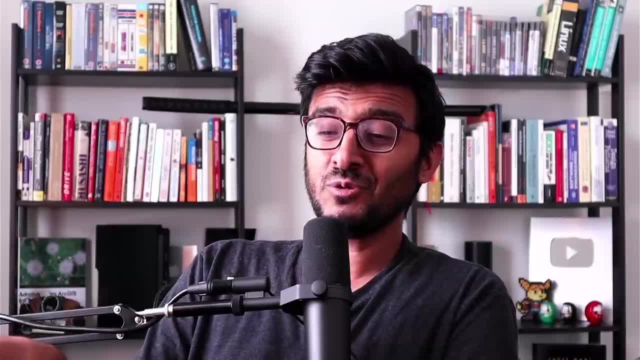 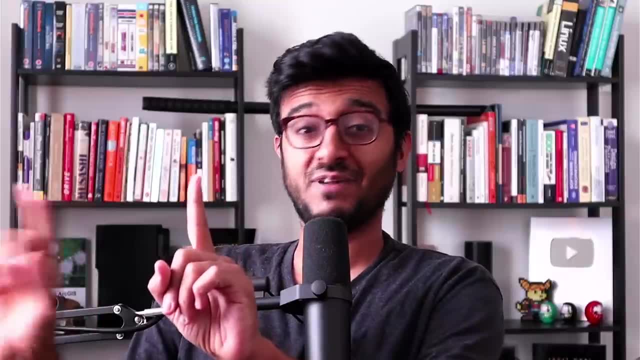 But a single IO will give you, if you think about it, repeated stuff. right, Because it's going to give you one and it's going to give you, uh, the value, and then another one, which is you, and then the value one three. 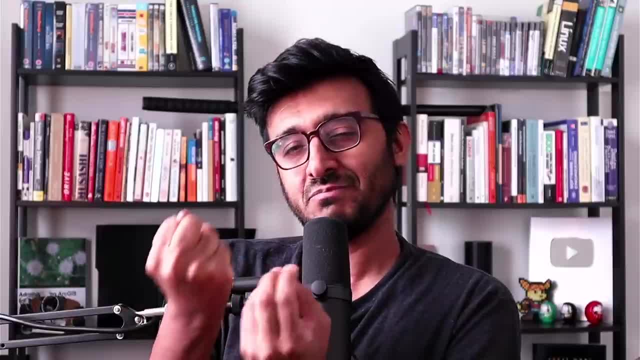 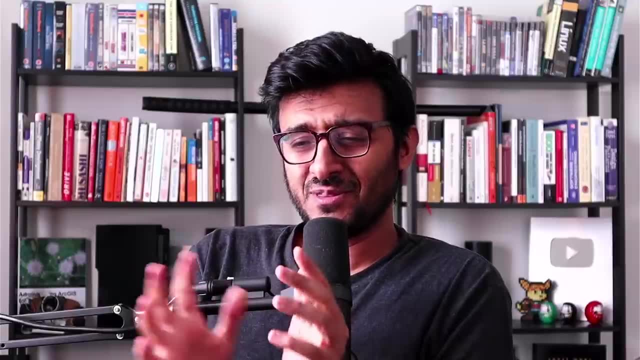 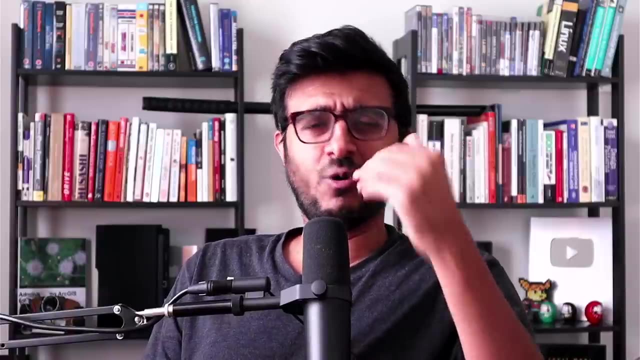 So there is some duplication, So you're wasting precious bits storing it when you don't really need to. And not only that, by the way, there is the fragmentation that can happen because- guess what? That when, when I'm your friend, like one is a friend of two and one is friend of three. 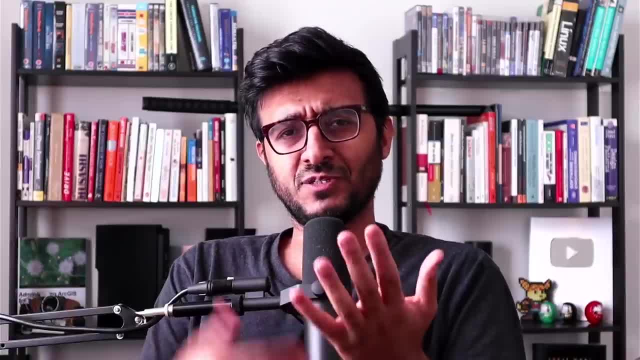 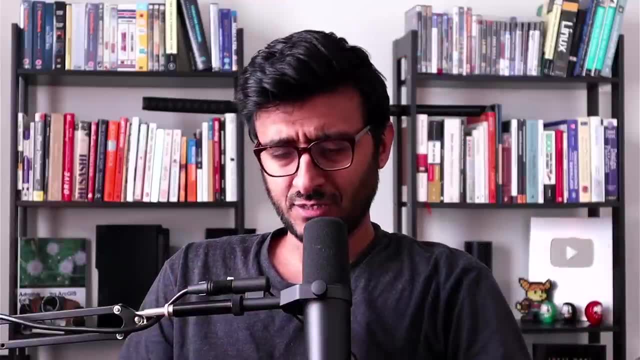 and one is friend four, right, And then two is friend of five and two is friend of six- right. Then the data will be stored in a homogenized manner, right? This is how the data is stored. It's not like ordered or anything like that, right. 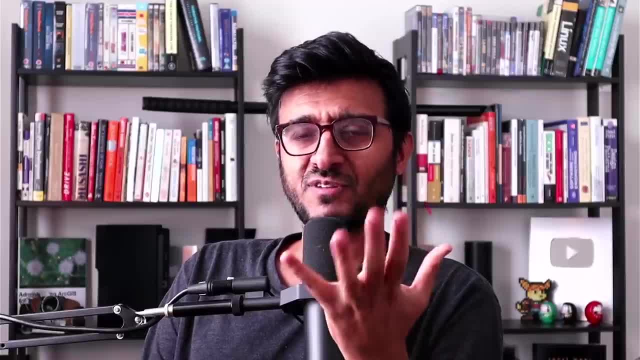 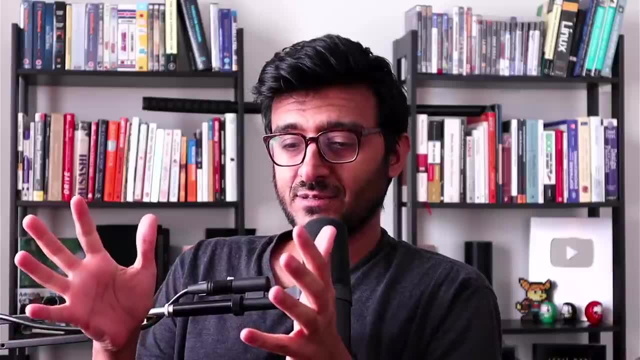 So, when you want to find my friends, like all the friends for the ID number one, not only you going to give, You're going to do a read, You're going to, not only you're going to get your friends, you're going to get other. 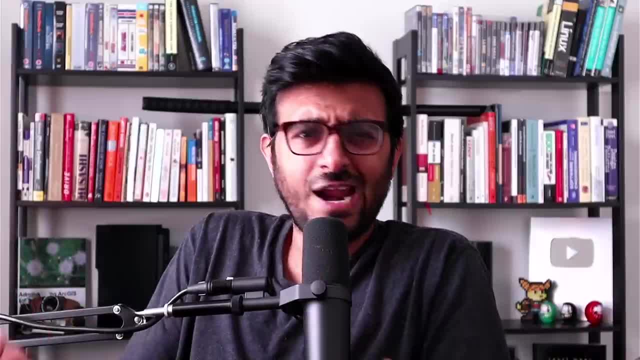 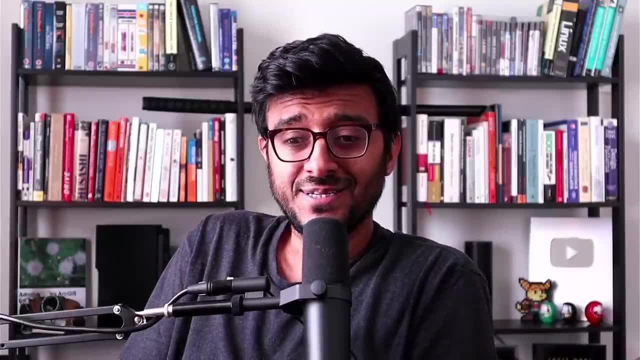 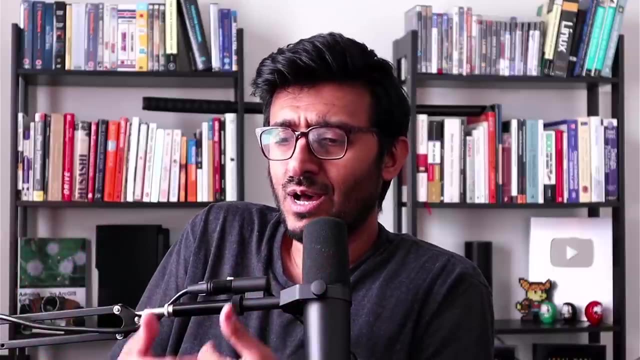 others, friends, because the data is just stored randomly, right? There is no order to the, to the actual table, right? So it's just stored this way And the result you get you're going to have to, you know, look through a bunch of stuff. 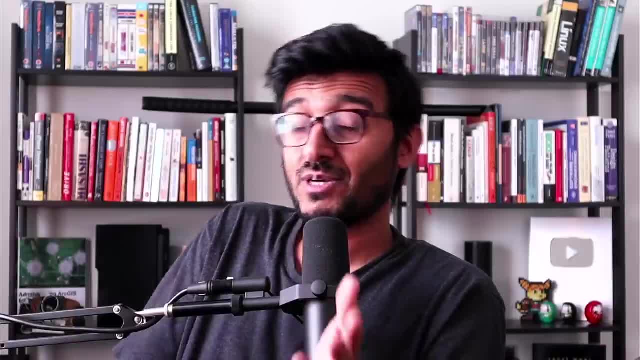 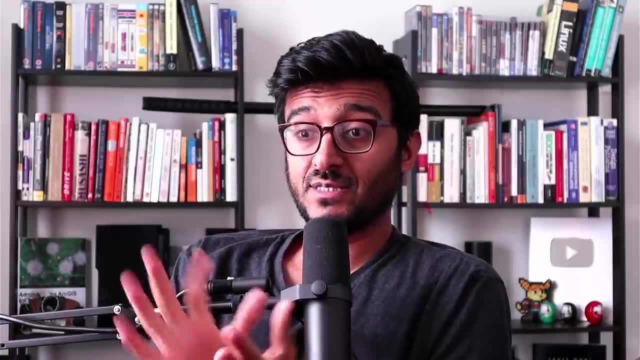 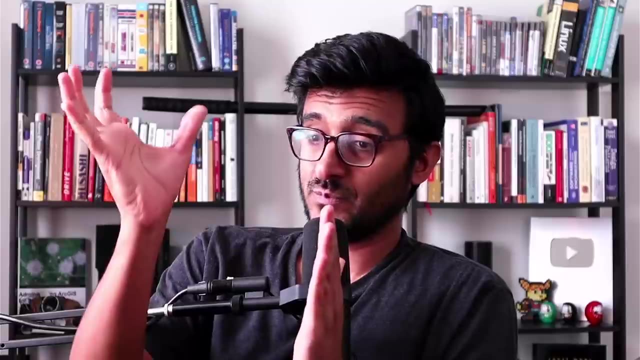 that you don't want, And that's the cost comes back to the cost You might say I want to. I can cluster my table by by the ID. this way, If I cluster by the brand ID, then if I cluster by ID, then all the data will be exactly ordered. 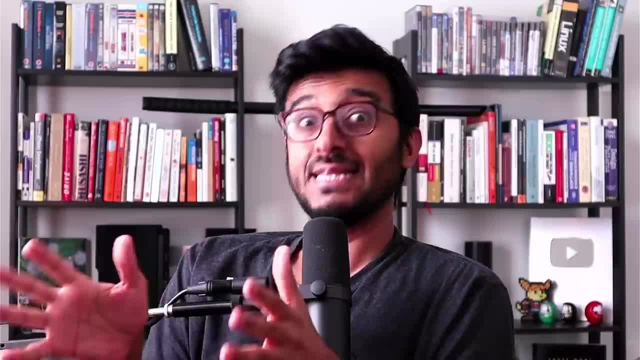 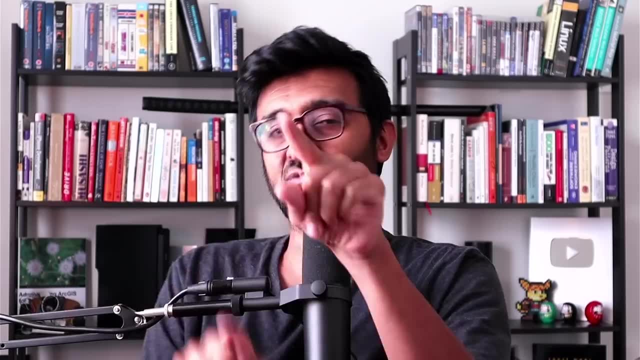 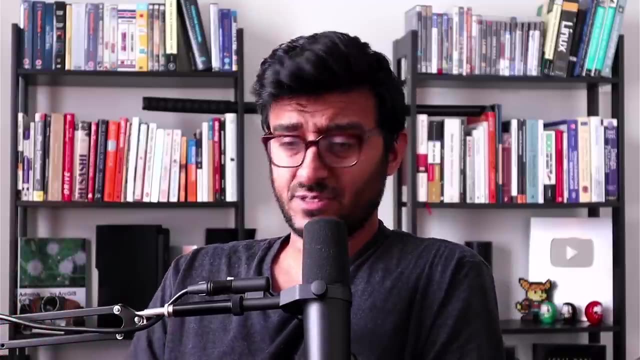 and organized in the disc in that manner. That obviously will be costly, because insert will be slightly slower because now I have to find exactly where to insert the data. Right, But that's effectively it. You can definitely build it and you can add indexes to optimize the queries. 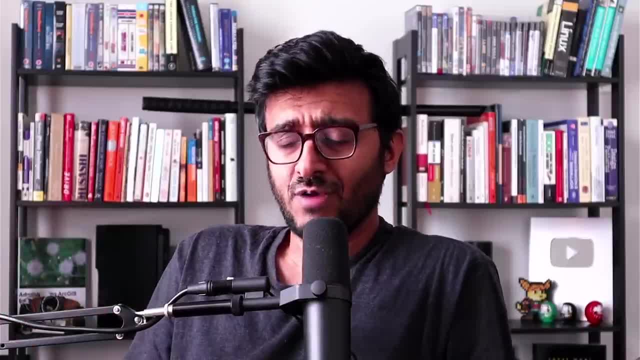 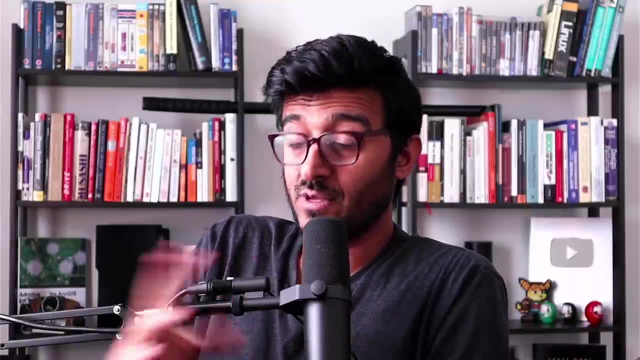 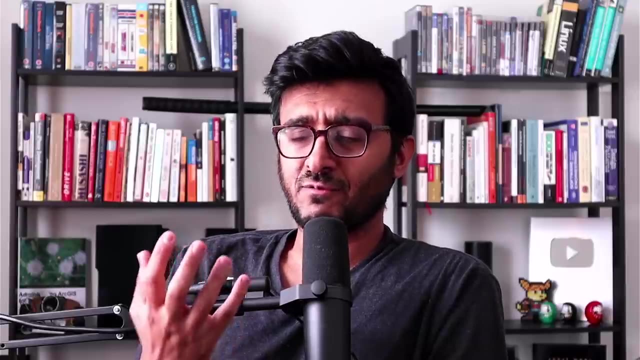 Nothing wrong with that. You can do so many tricks, but the graph databases come into the picture to make that even better. So you can think about the things that you can build with the graph databases. right, You can your. first of all, you have to build a brand new graph storage. 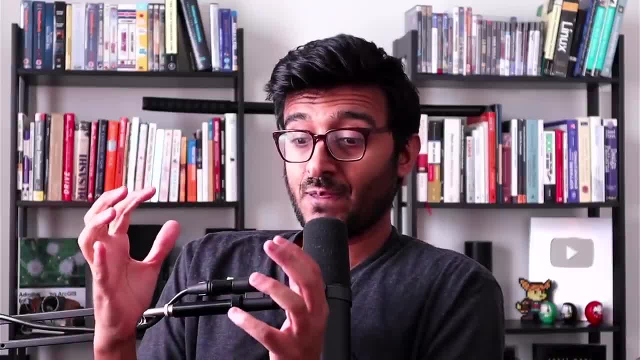 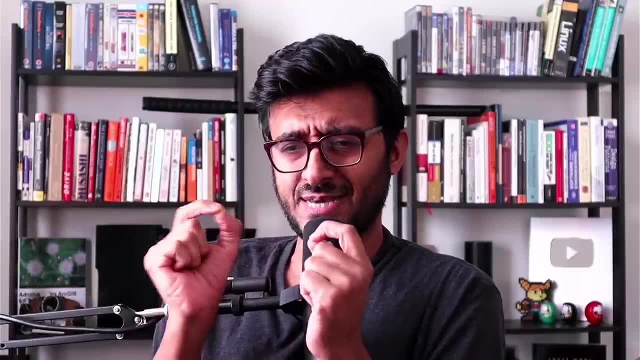 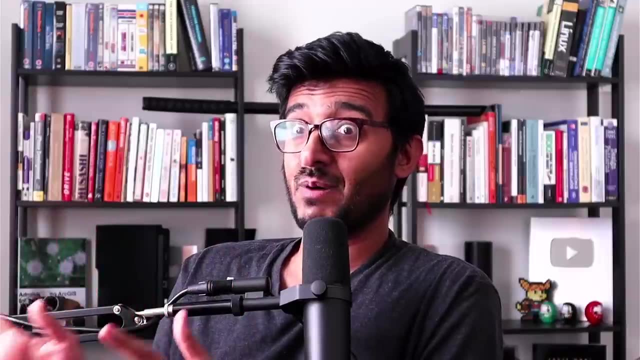 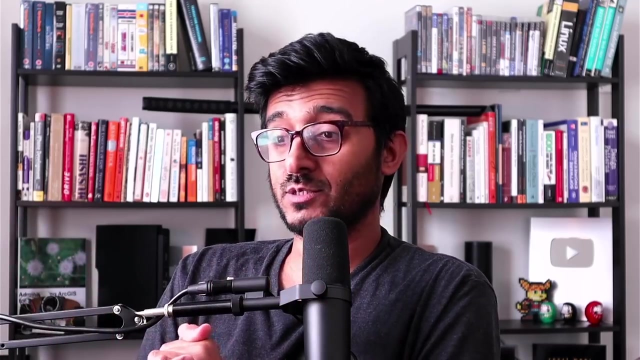 So that it is optimized to store graph data. The graph data is usually very, very tiny, like the actual node IDs. You can store them in the traversal and you can have the actual data about the nodes, Like what is the node name or I don't know if there is metadata associated with the node. 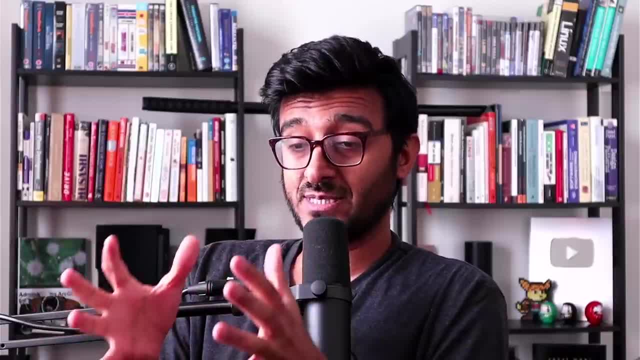 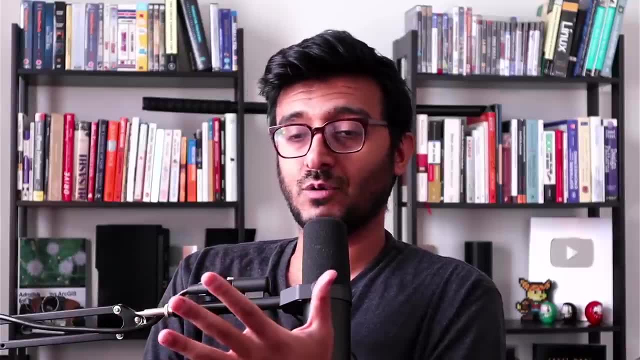 You can put it some other place. so you can put a basic data structure, Okay, For the, for the storage of the graph itself. All right, Now how is it stored? And you can put another data structure to store the metadata about the nodes. 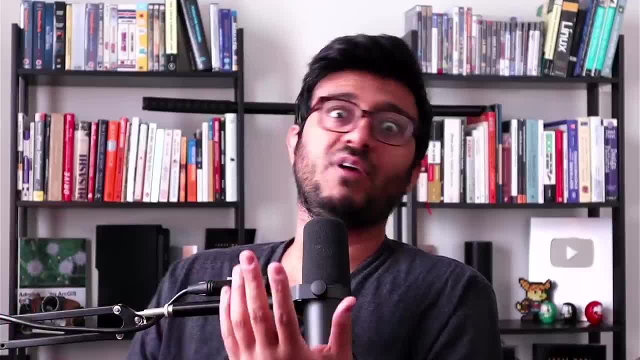 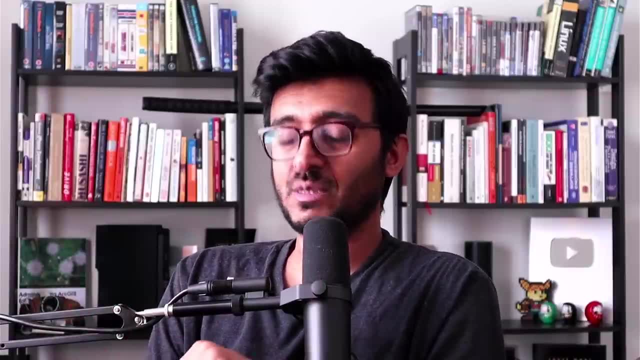 You know heavy stuff there: Profile, lecture and stuff. And not only that. I can see a lot of optimization that you can do at the indexes structure. Build a brand new index data structure that allows you to do not only breadth first, but 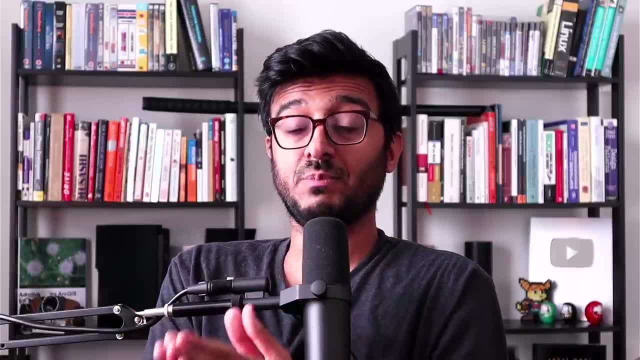 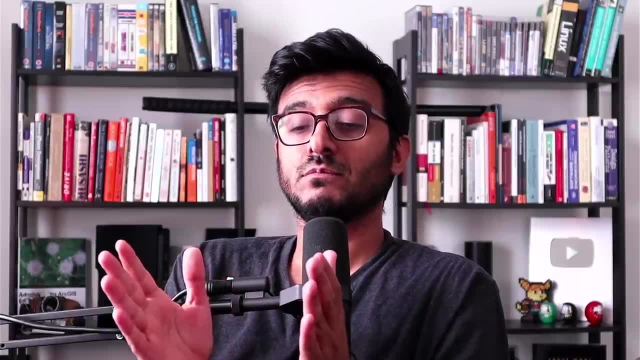 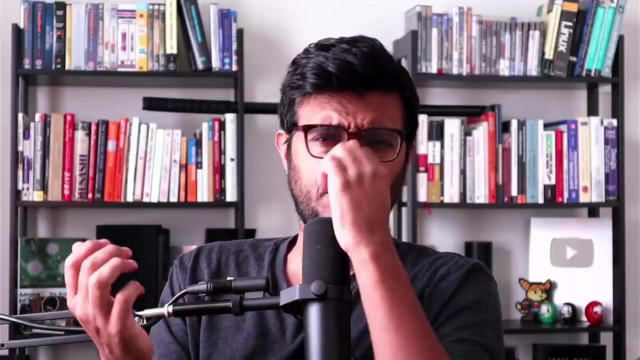 also depth first index. So if you're doing depth first go to this index, If you're doing breadth first, go to this index And, as a result, I can see why graph databases are are being built. There are many of them. 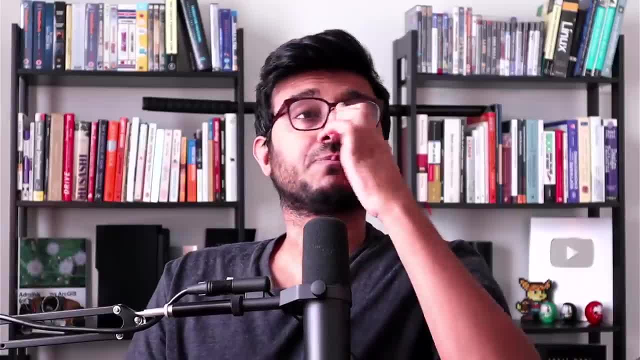 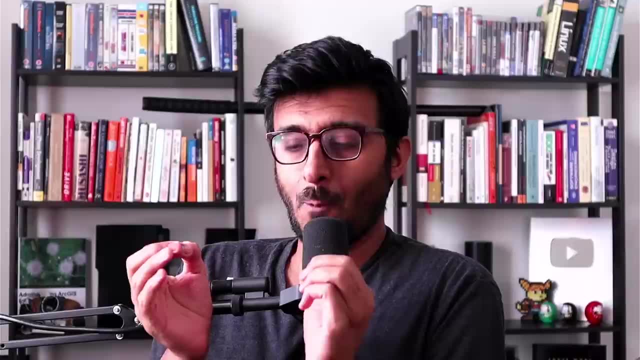 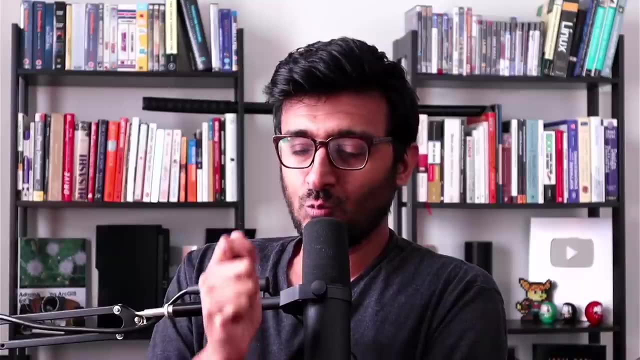 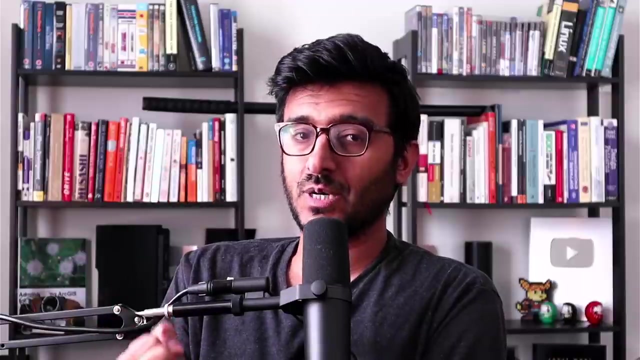 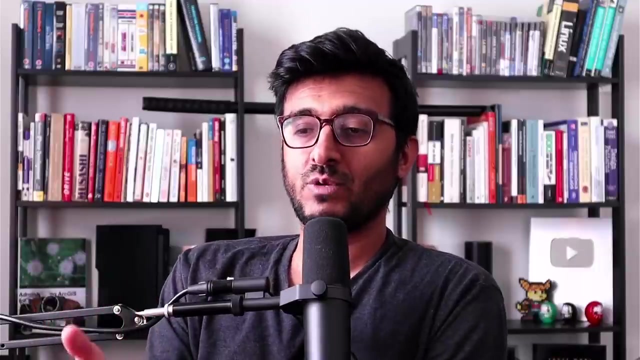 So definitely they are critical. So, to summarize, I think it always comes down to your use case. I believe if you really know, um, how the database works internally and what a single IO from desk gives you back, you can really optimize the heck out of every single costly IO so that when it comes back, 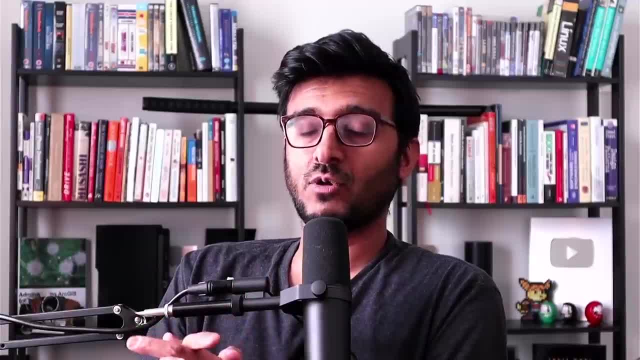 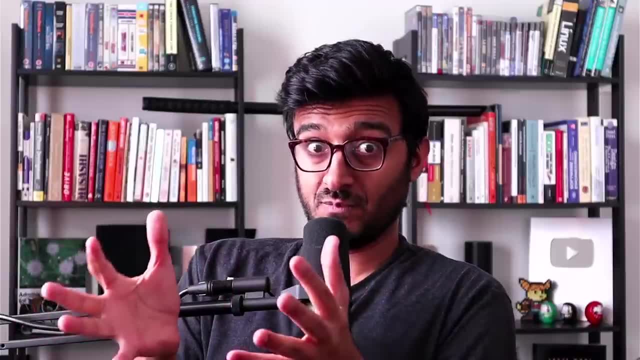 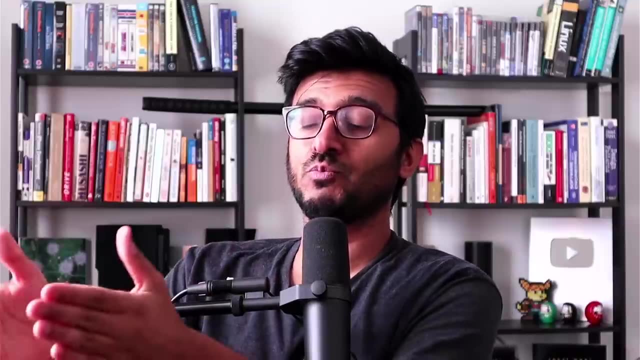 it got everything you need and you ask it for. So if you ask for, uh, the graph traversal all the values that you got from The desk, you don't really need to do much processing. You are not forced to go back to desk to fetch more blocks to get the data right. 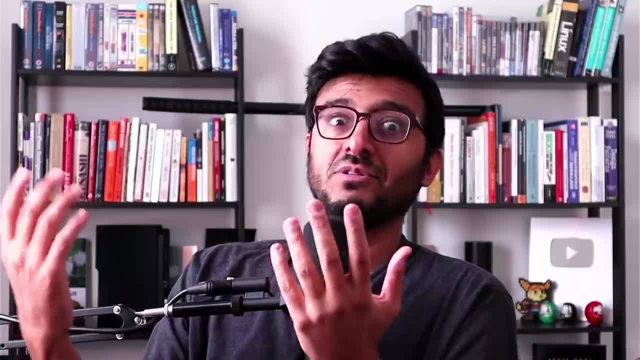 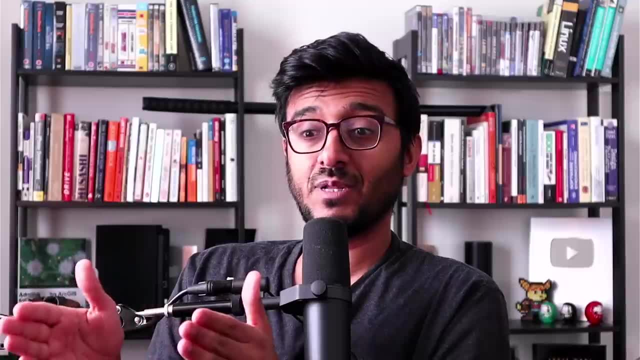 Obviously, most of the queries won't be satisfied with single IO. That would be awesome if you can, right, But if if you can't, then you can do multiple IOs. but the the less IOs you do and the 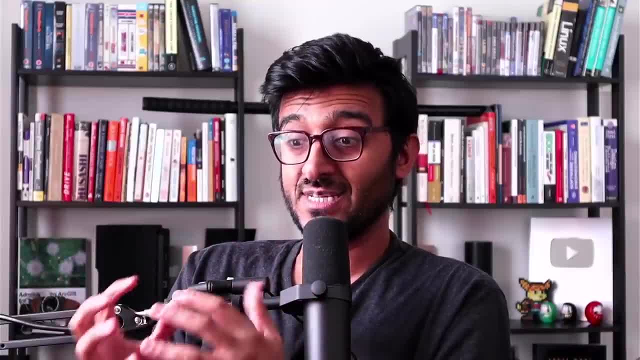 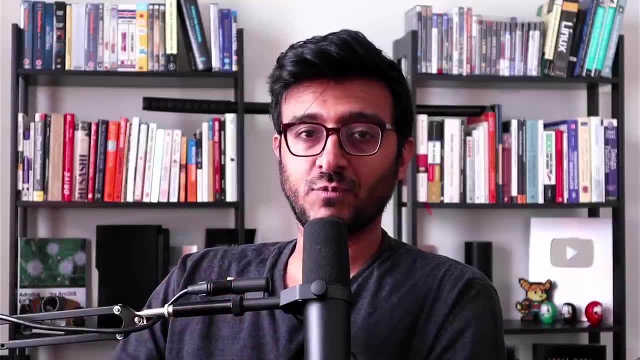 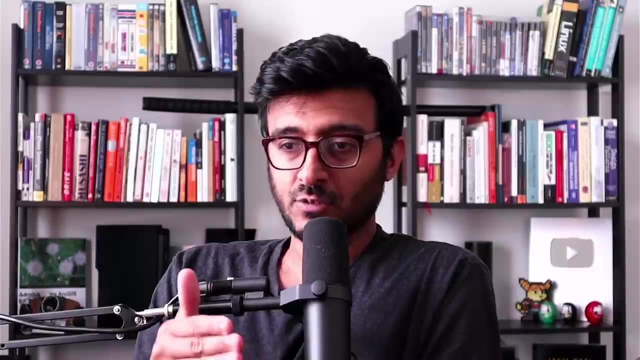 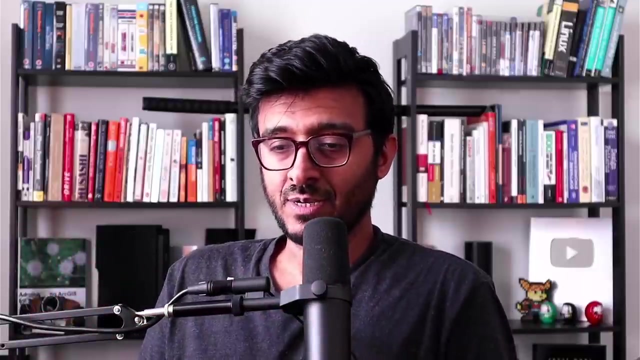 more data you get, Okay, The more data that you get is effectively exactly what you need. That is where what you want to build effectively- And that's really all what matters. The algorithms obviously plays a role at the application side. How do you process the data?